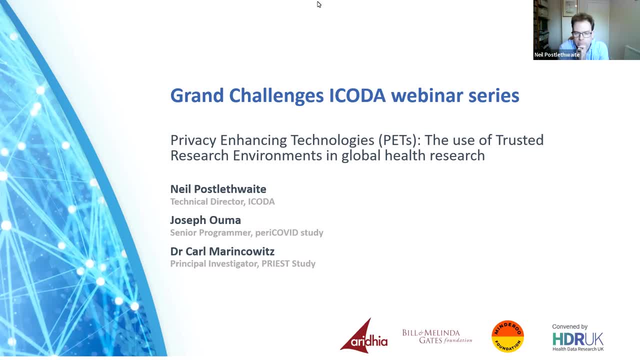 All right. Well, we are at a couple of minutes past the hour, So let's jump in. Firstly, a very warm welcome to the next in this sequence of ICODA Grand Challenges webinars And thank you for spending the time with us today, And we've covered a number of topics in these. 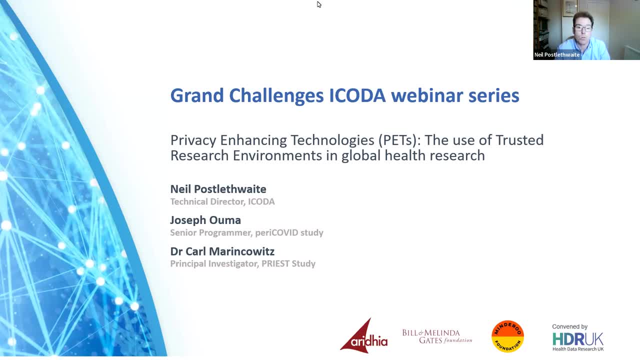 webinars so far in the series, from some of the individual driver projects to topics such as natural language processing. All of the replays of the sessions are available from ICODA's website, So do take a moment or two to go and have a look through some of those. 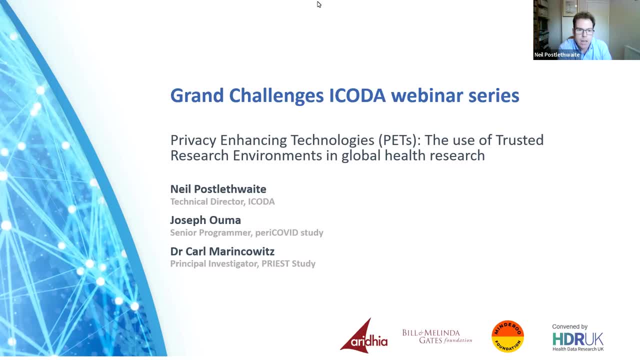 Would be excellent. Today, we are going to cover privacy and enhancing technologies, with a specific focus on trusted research environments, So privacy enhancing technologies, or PETs as they are more affectionately known. I'm privileged to be joined today by Joseph Uma, who's the senior programmer in one of the ICODA projects. 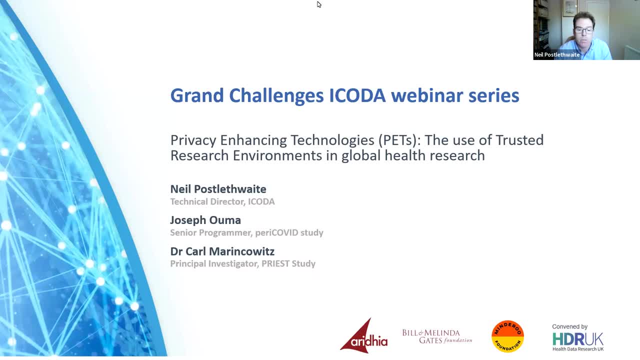 the PERI-COVID study and also Dr Karl Marinkovits from the PRIEST study. So they join us from the Makera Johns Hopkins University in Uganda And Sheffield University here in the UK. So delighted to have them with us And I'll take 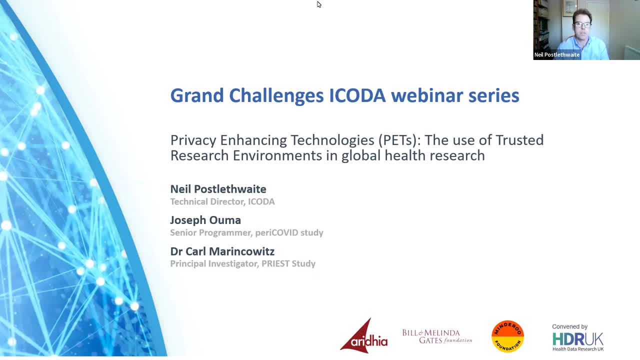 you through the agenda in a moment. Just a couple of bits of housekeeping as well, And today's session is being recorded, So just be aware. And also, please put any questions that you have for myself or the other presenters in the Q&A section for the webinar rather than the chat. Okay, 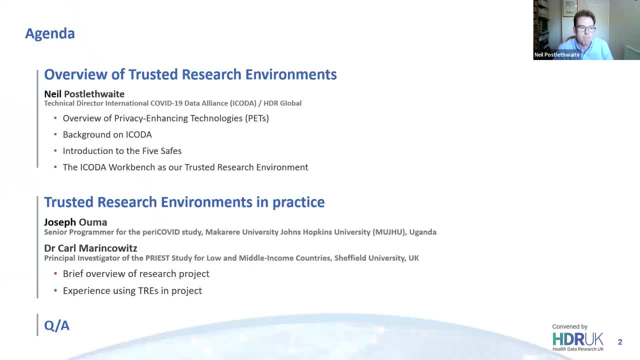 hopefully that makes sense, So let's jump in. So the agenda for today is a bit of an overview of privacy enhancing technologies, trusted research environments, a bit of background on the international COVID-19 data alliance, ICODA, for which I'm technical director, And then the far more interesting and 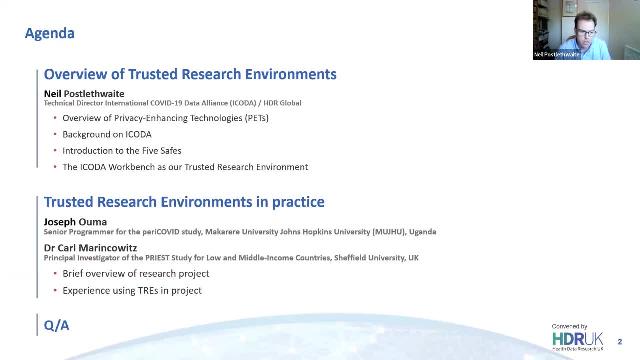 exciting piece of the webinar will kick off when Joseph and Karl will take you through an overview of their research projects and their experiences using trusted research environments within those projects. So we'll each aim to do about 15 minutes, As I say. please put questions. 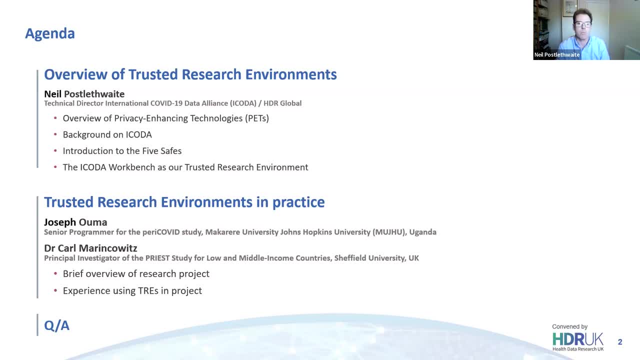 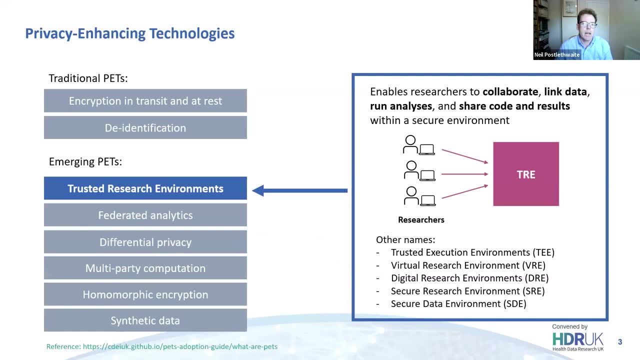 in the Q&A box as we go along And we'll save some time for those at the end. So let's make a start with privacy enhancing technologies. So I think firstly important to think about what do we mean by privacy enhancing technologies? What kind of thing are we talking? 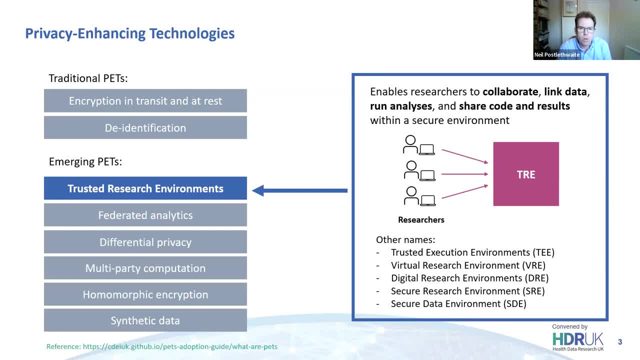 about here, And these are technologies really aimed at enabling data protection and minimising use of personal data. So this is all about protecting both your personal data, my personal data- and anybody else who's part of a cohort, And this is especially key in health data research. 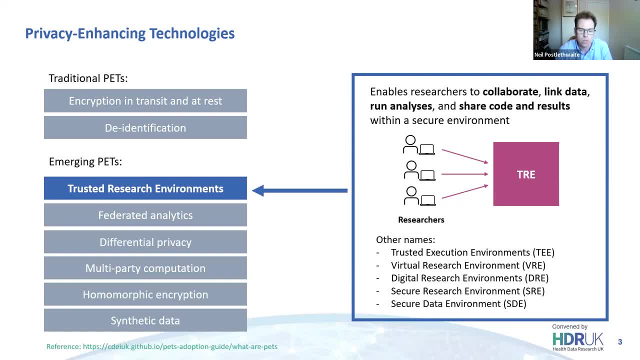 To protect our privacy as patients or as part of those cohorts. And traditionally I think if you look at the at the top couple of boxes, the first thing that we think about with privacy enhancing technologies in a traditional sense is encryption. So encrypt the data. So if somebody inadvertently 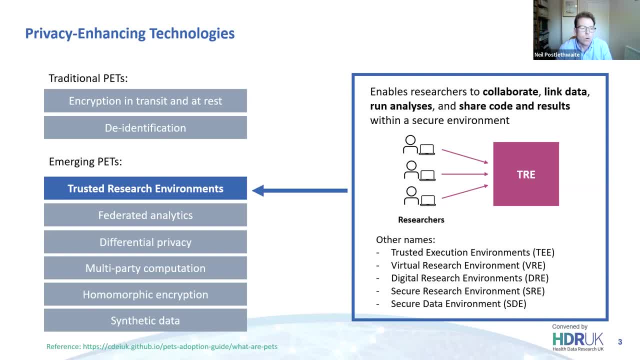 gets it, they can't access it and read it. Or de-identification, So removing identifiable information, information from data, So that might be things like your name, your date of birth, a localised address, something like that, and replacing it with some kind of ID or token So you still have. 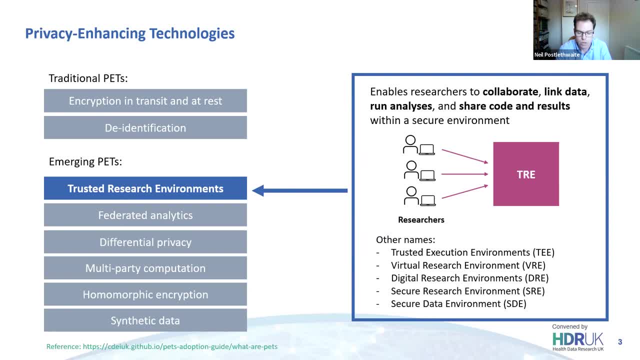 the data, but you don't know who that data belongs to. We have a new set of what we call emerging privacy enhancing technologies, of which trusted research environments that we're going to talk to today are an example of, But we also have some other things that are gradually coming to the 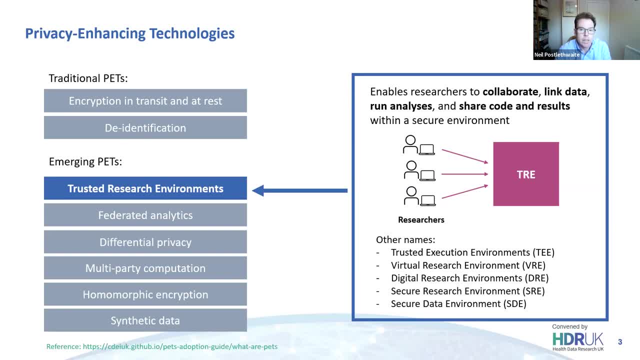 fore. So federated analysis, where the data doesn't move. So data would remain in a single repository and researchers would send access requests to that data and results would be returned. Differential privacy: So that's where algorithms actually don't know if particular. 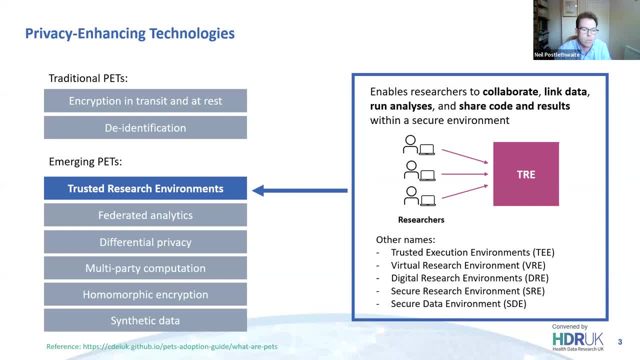 individuals are in a particular repository. So that's where algorithms actually don't know if individuals are in a particular repository. So that's where algorithms actually don't know if individuals are in results sets, So very difficult to ascertain or identify an individual using differential privacy- Things like homomorphic encryption, where analysis is actually run on. 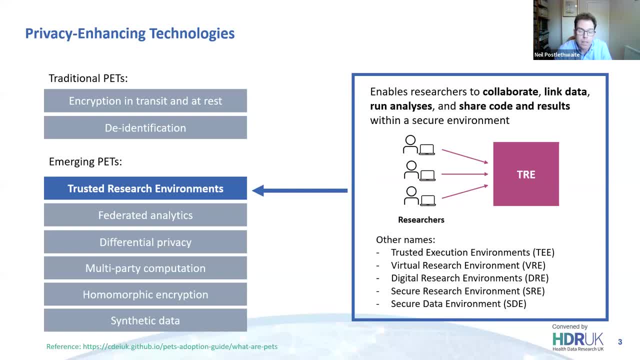 encrypted data and synthetic data, where data is artificially generated based on algorithms and models. So there's no silver bullet here in terms of data protection. this is really a continuum, And I think it's important to understand. the more that we obfuscate things and the more we make things completely unidentifiable, often the less useful that data is from a research perspective in terms of actually answering a specific question. 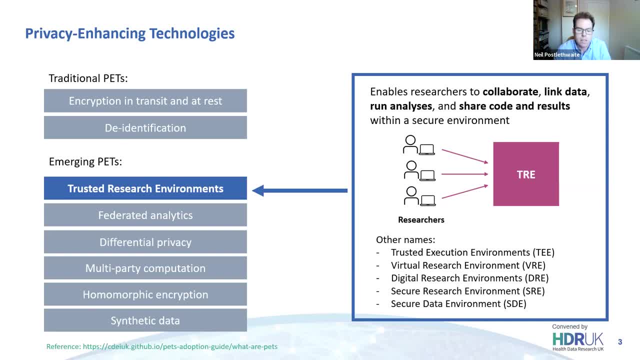 But I think the important thing to understand is this is a continuum and quite often a blend of these privacy enhancing technologies is able to achieve a good balance of both research usefulness and protecting the individual. So you'll hear trusted research environments, which we're going to focus on today, referred to by other things as well. 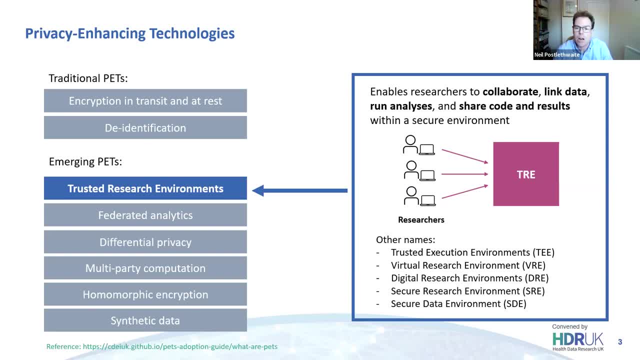 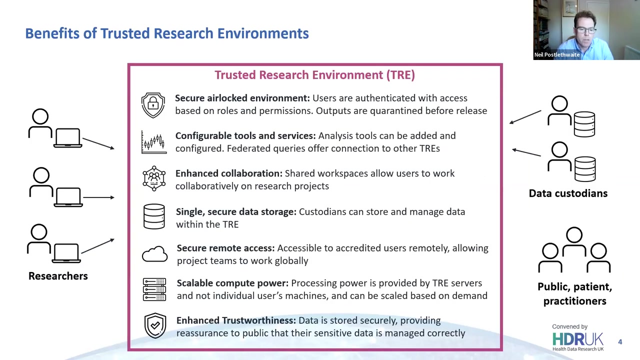 So we use the trusted research environments TRE. TRE is the typical acronym. You'll hear virtual research environments, digital research environments, secure research environments, secure data environments- It's all effectively the same concept under slightly different names. So what do we mean by a trusted research environment and what are some of the characteristics? 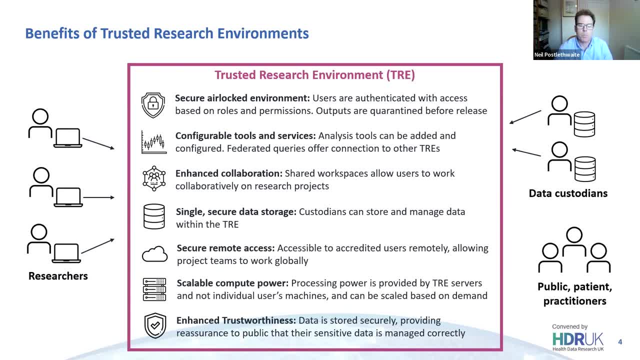 So typically, a trusted research environment provides a set of things like An airlocked environment, So any user accessing a trusted research environment is authenticated, often pre-authenticated, and their researcher accreditation is assessed before they're even allowed to go towards log on. 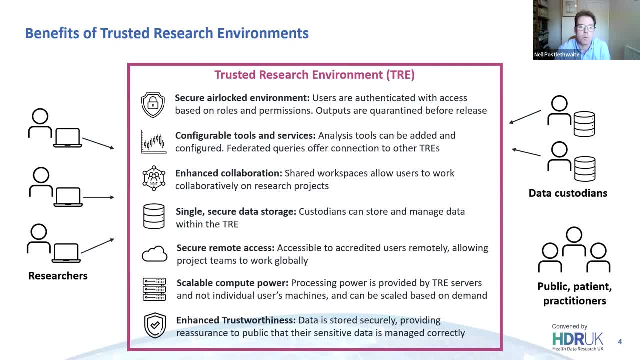 They're not allowed to take anything out of a trusted research environment without it going through quarantine and making sure there's nothing identifiable in that output. Usually they have a set of configurable tools and services, So tools within which you can do analysis, and typically they can be added as well. 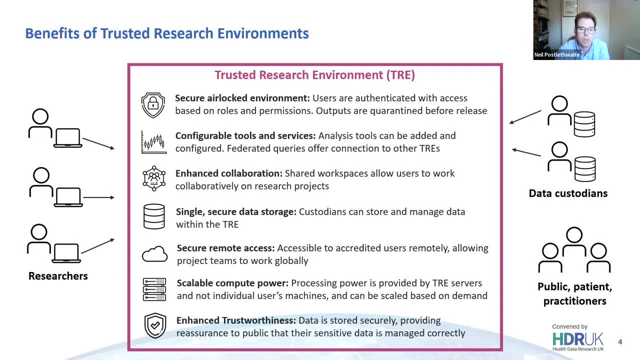 And most trusted research environments will allow you to add and configure tools and services- and they're really there- so that a research team can work in a secure collaborative environment on a set of data provisioned into that trusted research environment by a data custodian. 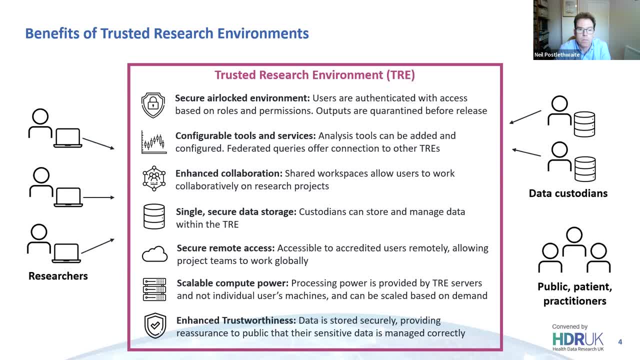 So it does save very much the having multiple copies of data With lots and lots of researchers as well. Typically they're available remotely and quite often with cloud access as well, which has been particularly useful in the international COVID-19 data alliance with researchers all over the globe. 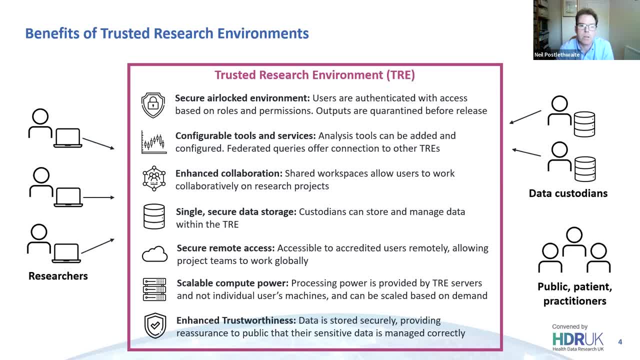 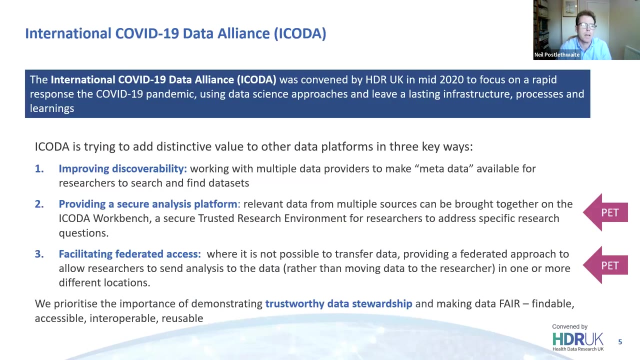 Very often it's straightforward to add more computing power to a trusted research environment. so if you are needing to do a particular analysis or run particularly intensive algorithms, you can add virtual machines to the environment. This is under the. So that's some of the benefits. 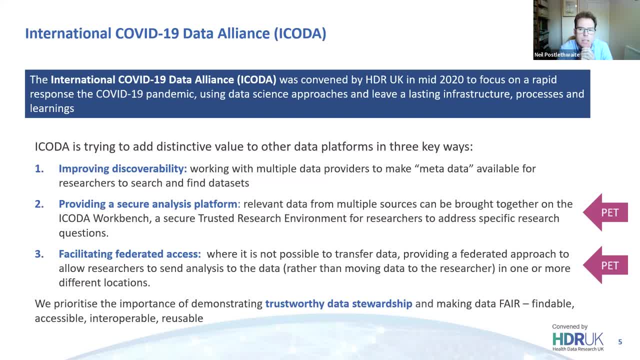 Just stepping back a little bit and looking at the iCODA initiative. The iCODA initiative was convened midway through 2020, really to convene a rapid response to the COVID-19 pandemic. you're hearing from today as well are in the the wrap-up phase of the initiative. it's important. 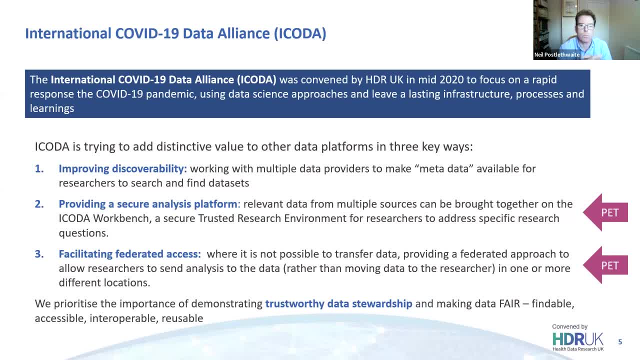 that we capture all of the learnings for that, and you will see more and more publications and outputs from the initiative as we go over the next couple of months. we've tried to do things a little bit differently. we've tried to focus on making sure that data is fair, so findable. 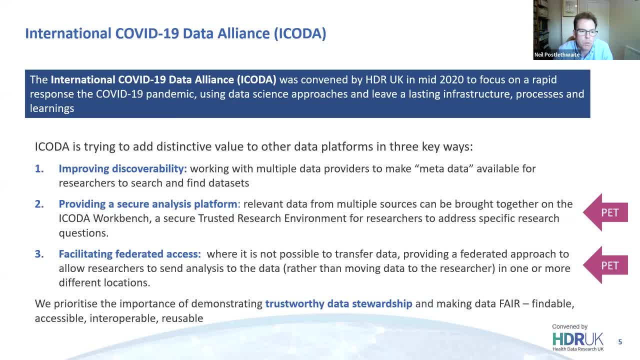 accessible, interoperable, reusable and discoverable in a very open fashion. all of our projects have run within a secure analysis platform- our trusted research environment, the icoda workbench, so a privacy enhancing technology, and some of the projects have been using federated analysis as well, so they've actually been sending analysis requests to the data from our trusted research. 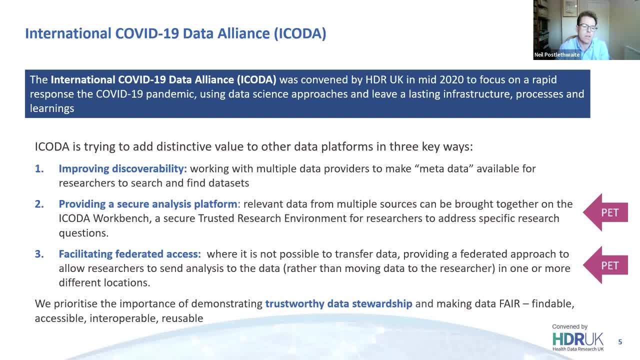 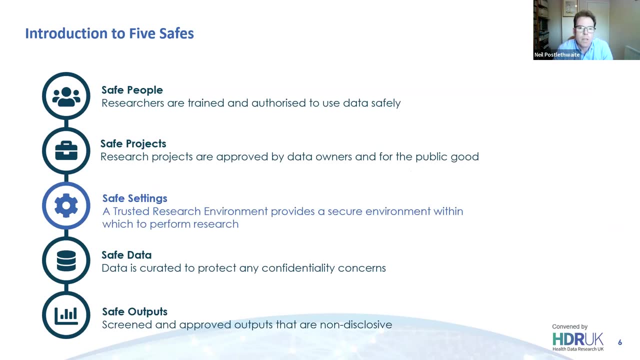 environment to another environment and having the analysis results come back, and we've really focused on trustworthy data stewardship. through the initiative. we've used a concept called the five safes in the in the background for the whole project. this is a concept that was brought together by the uk's office of national statistics, the ons, and it. 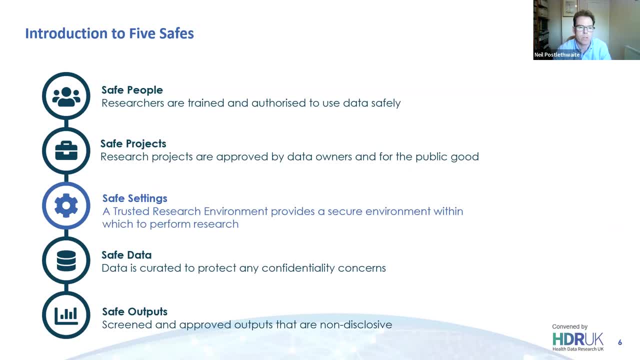 focuses on five categories. so safe people: making sure that researchers are trained and authorized and have appropriate accreditation to access data. safe projects: making sure that all projects are approved and are in public benefit. the projects are done within a safe setting. so the trusted research environments we're talking. 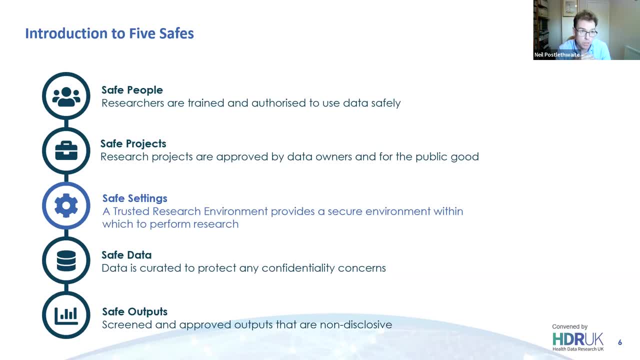 about today. data is curated safely, so the majority of the icoda projects have been working with either de-identified or summary level data. so no identifiable personal data within our project set and all outputs have been screened to ensure that there is no disclosive information in those. 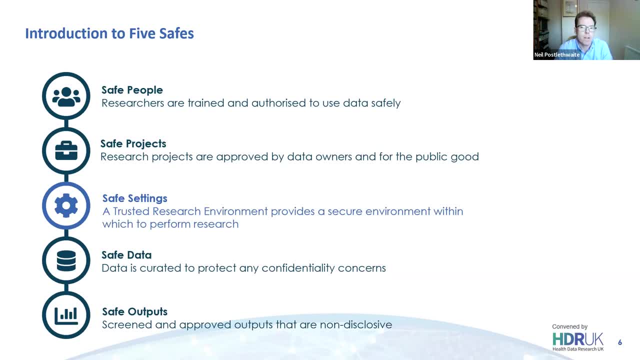 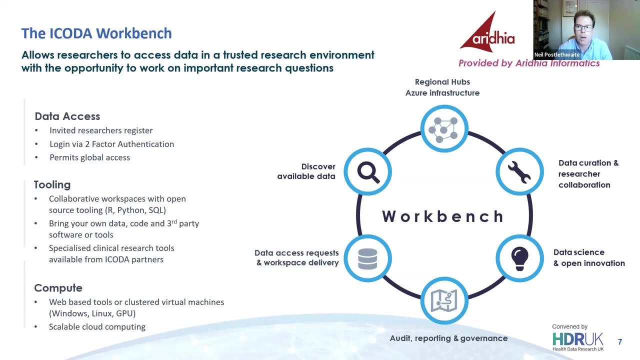 outputs. so those five safes provide a really nice lens within which to review health data research. the icoda workbench itself, our trusted research environment, is provided by our partner, iridia informatics. the workbench is cloud hosted on the microsoft azure cloud platform, and the aridia team have been able to stand the workbench up in multiple 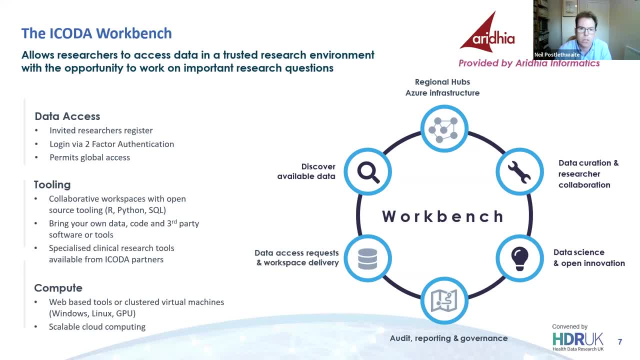 different cloud data centers across the world. for us as part of the icoder initiative, which has been fantastic. the workbench provides a secure two-factor authentication for researchers to log on a collaborative working space with open tooling. but other tools, other tools can be added and a number of our projects have actually had tools added to their workspaces you can bring. 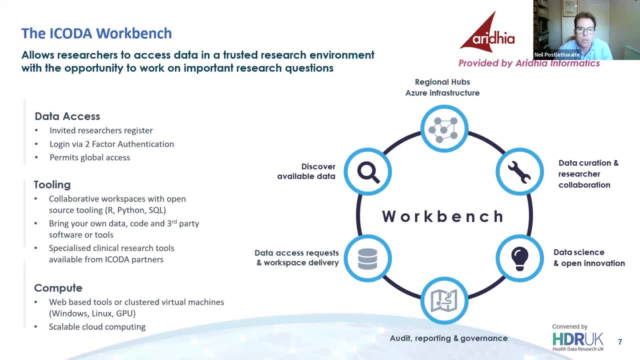 your own code and third-party software tools as well. you can add in compute power, which a number of projects have needed for particularly weighty analyses. you can add in virtual machines in either a win, windows or linux form, and also a set of metadata services has been provided, which is 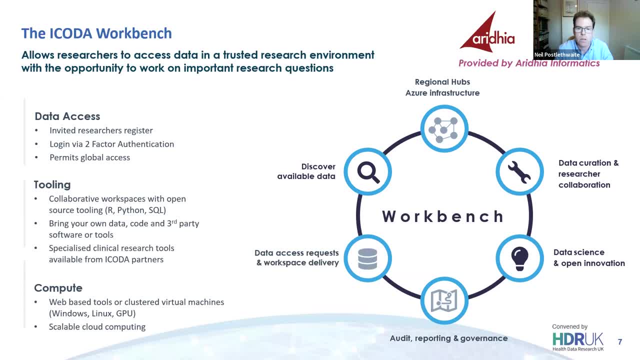 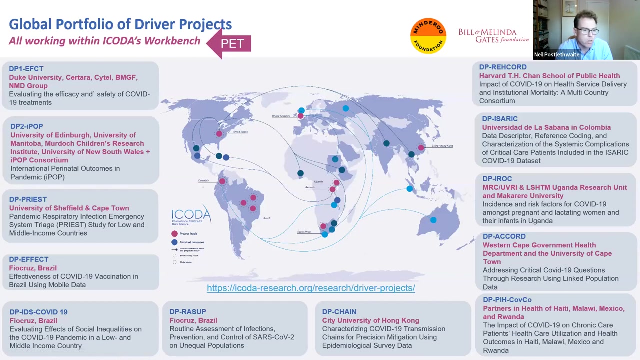 part of the icoder initiative, which we've integrated with our icoder gateway to make sure that all of the metadata in the project is available in a findable, accessible, interoperable, reusable fashion. so that's where all of our projects have been working. we've had a global portfolio of projects, two of two of which are with you today, but we've 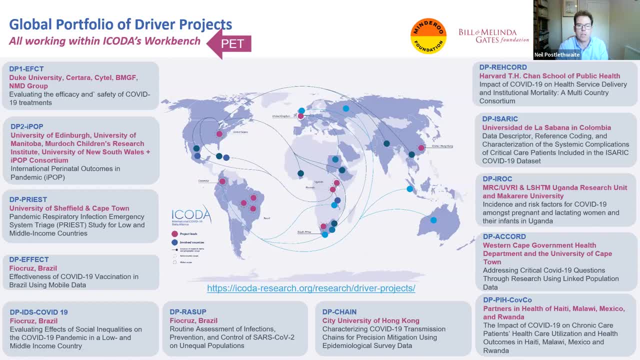 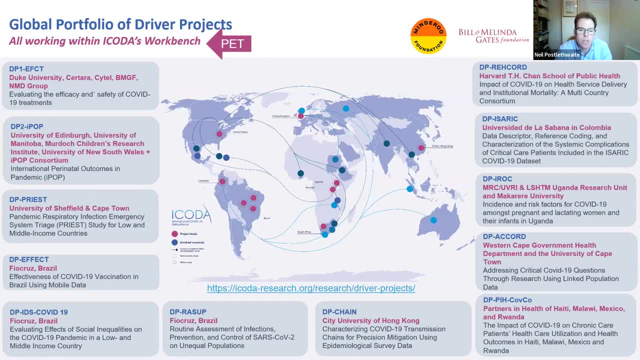 pandemic has affected health service delivery across multiple countries, so it's been our absolute privilege to be involved with all of these 12 projects all around the world. it's been a fantastic set of researchers and they've made some really good use of of the tools that have. 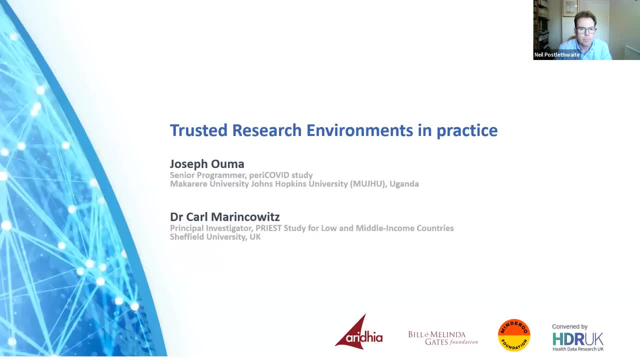 been provided as part of the initiative. so i think with that, that's hopefully sets the scene in terms of a little bit about privacy enhancing technologies, a little bit about trusted research environments and some of their characteristics. i'd like to pass the baton over now to firstly joseph and and then carl to take. 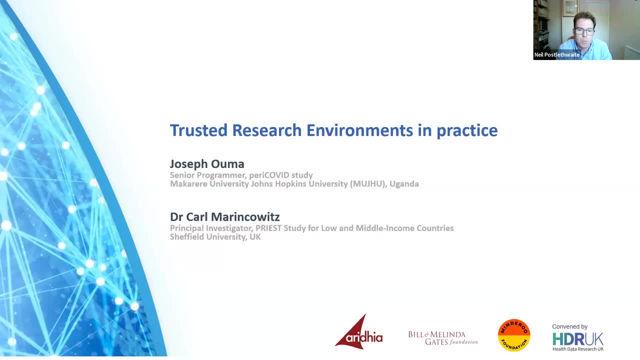 you through a little bit about their projects and how they've they've learned and used trusted research environments in in practice as well. so thank you very much. thank you very much, joseph. i'm going to stop sharing and, joseph, i'm going to pass the baton. 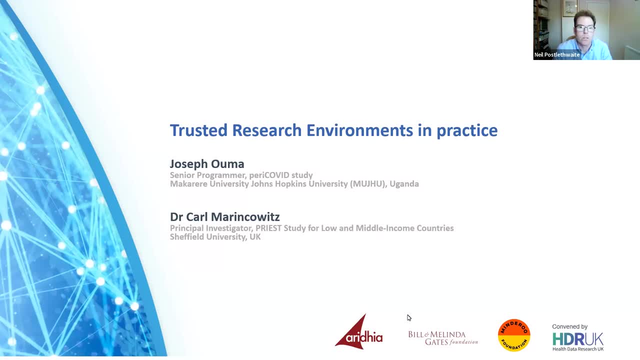 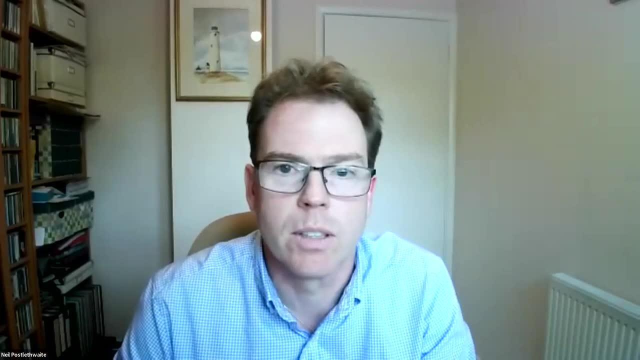 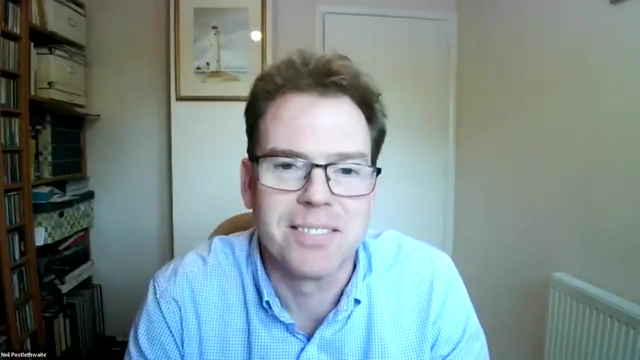 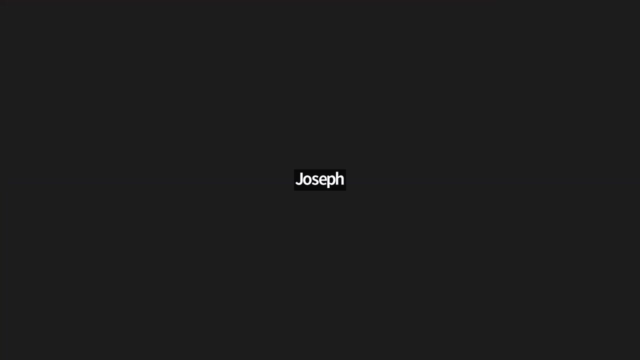 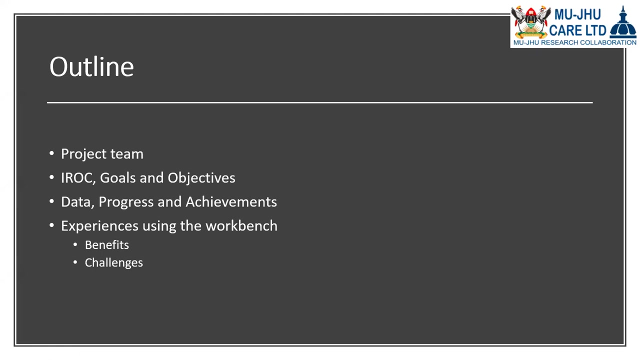 over to you, joseph. joseph, you're on mute. oh, hi, Neil, thank you, i'm just trying to keep my slide up. that's all right. thank you, all right, take your time, okay, and please see it now. i was bang on time at 15 minutes. yes, i can. 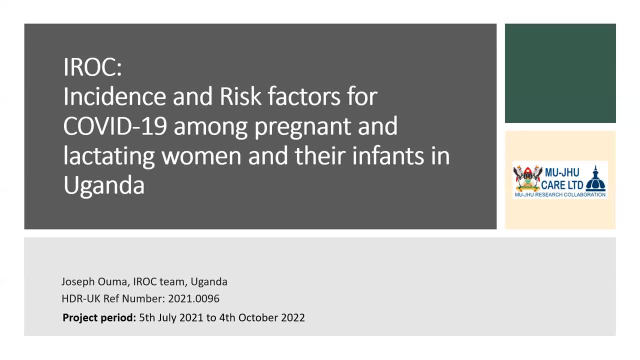 see your slides. take us away, okay, good, thank you very much, neil, and good afternoon, good morning to everyone. uh, thank you, uh and joseph, do you want to turn your camera on? there you go, yes, yes, thank you, thank you, and, um, just to say it again, good afternoon, good morning everyone, thank you all. 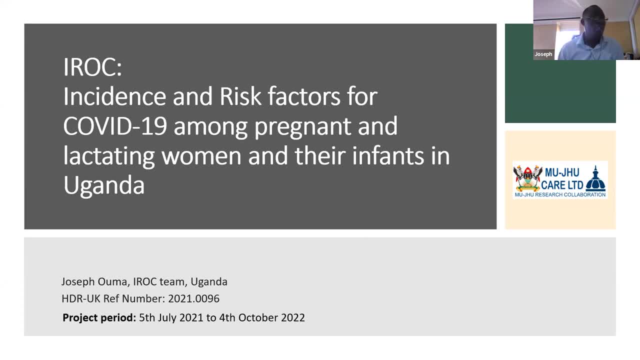 for making time to join the webinar this morning afternoon, wherever you are, and also thank you for the organizing team for inviting us to share our work and experiences using the iconda workbench. and, like neil mentioned, i'm joseph oma, the senior data manager and biostatistician here at muji. 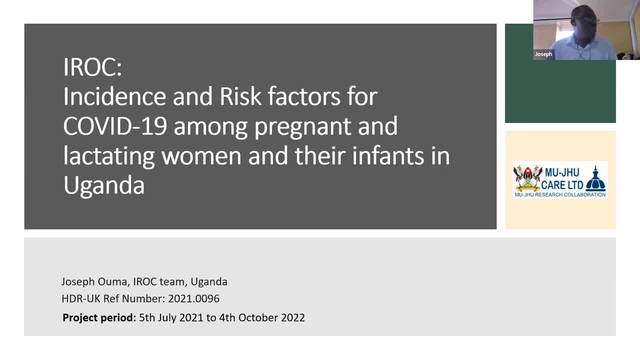 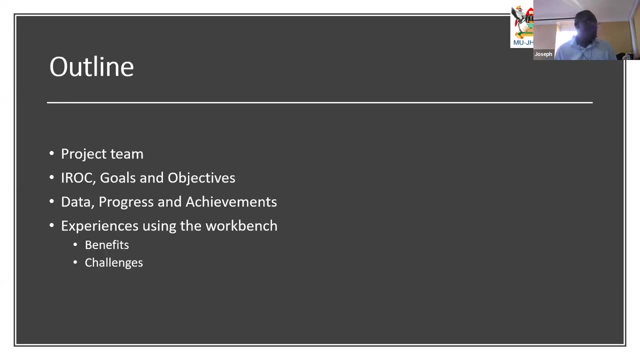 so i'm going to be talking to you about our project in uganda: the instance and research factors for covid 19 among pregnant and lactating women and their infants in uganda. um just to highlight what i'm going to be talking about, um i'll be presenting to our team. 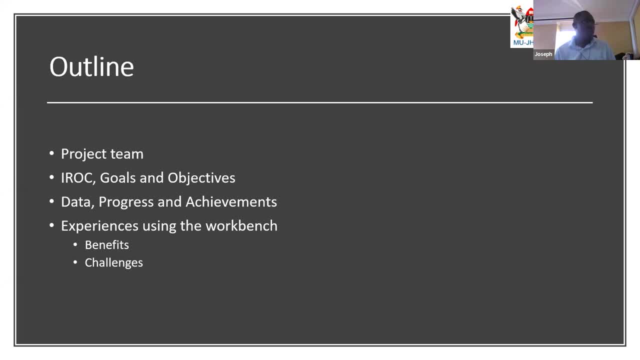 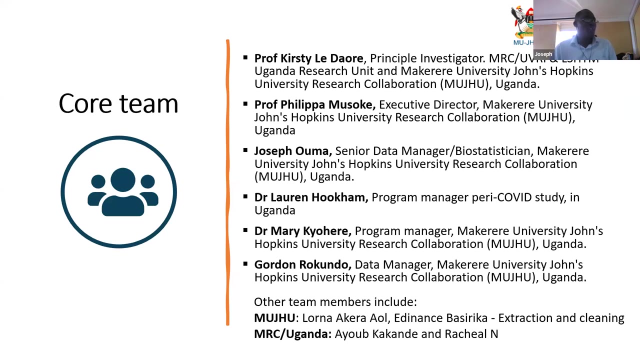 the goals and objectives of the project, the progress we've made and any achievements we've had so far, and our experiences using the iconda workbench. our team was led by professor kusty ladro. she was the principal investigator, and we also had the professor philippa who is the 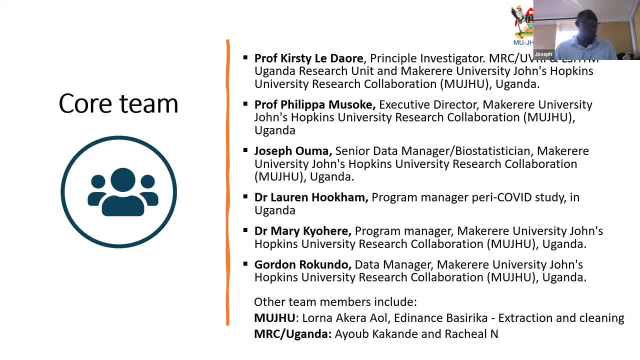 executive director of muji here in uganda, um myself and we also had clinical members of the team: dr laureen hookman, who was who was the program manager for pericomite and part of it i got our project. dr mary johira, we had gordon, who was in charge of our data management, and alona and edina, who 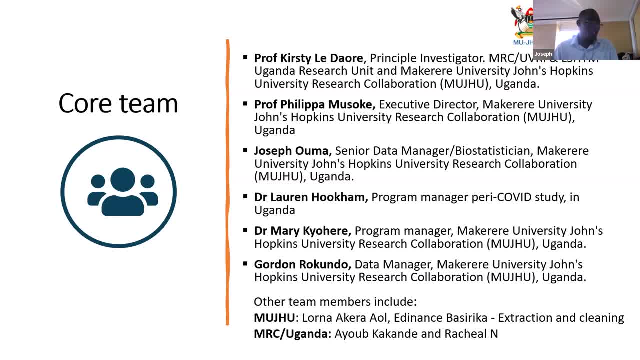 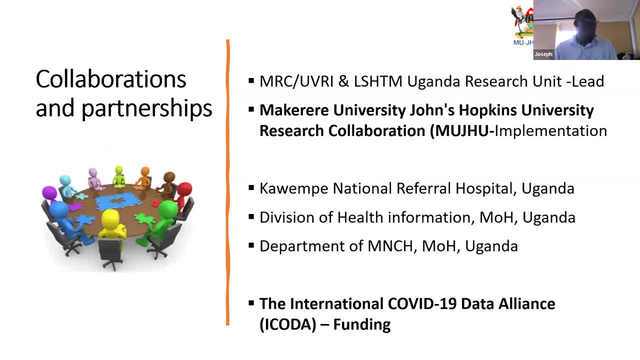 supported data extraction and cleaning, and we also had piu and rachel, who contributed to our work. in terms of the partnerships and collaborations, our work was led by mrc uvr as the lead institution. moju, which is the project manager of the project, is macquarie university. johns hopkins university research collaboration really has supported the 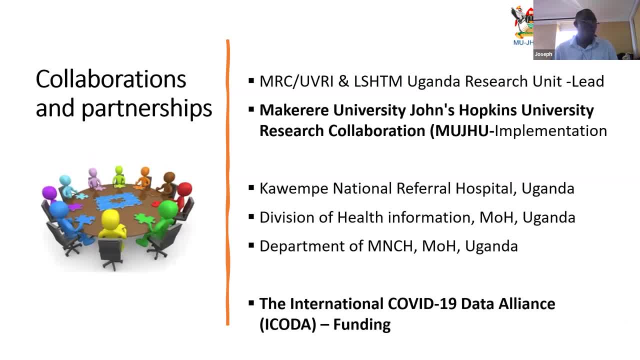 implementation uh. our other partners were kawinpe national referral hospital here in uganda, the division of health information uh minister of health in uganda, department of maternal and unitary child health in uganda and, of course i called the international copy 19 data allies. 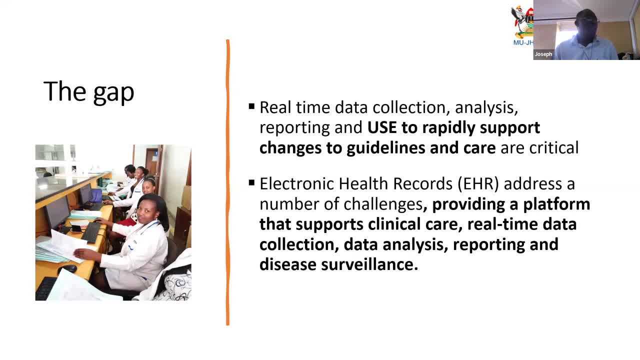 supported us with their funds? um at the inception. our project a gap? um. here we noted that real-time data collection, analysis and reporting are needed to support changes to guidelines and care, and therefore we thought that electronic health records provided this platform that's much needed to support this clinical care. 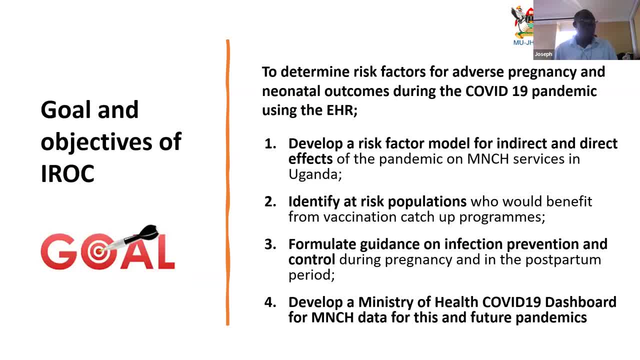 and disease surveillance. so therefore our project set out to be strategic: a risk factor model for indirect effects of COVID-19- sorry for the indirect and direct effects of the pandemic on maternal, neonatal and child health services in uganda. we also provided a Skid risk factors information on team core digital data. so we quickly recognized that because we had planned an 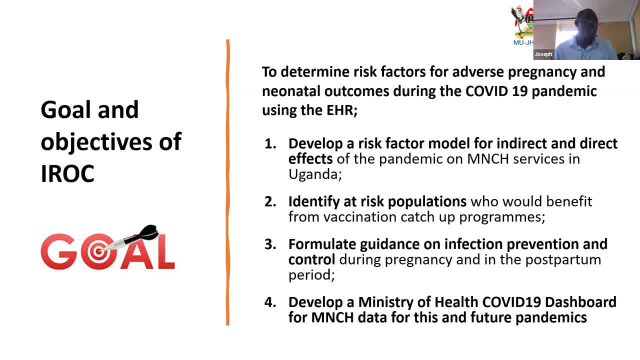 We wanted to identify the at-risk populations who would benefit from things like vaccination, catch-up programs after the closures or restrictions contain the epidemic or the pandemic. We also intended to formulate guidance on infection prevention and control during pregnancy and the postpartum period. And then, lastly, we wanted to develop a means of health- COVID-19 dashboard for maternal and neonatal child health data for this and future pandemics. 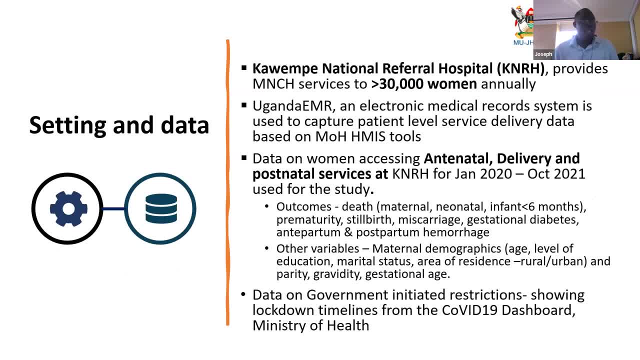 We used data from the Wempe National Repair Hospital, a maternal and neonatal child health facility providing services to more than 30,000 women annually here in Uganda. The hospital is located in the north of Uganda. The hospital uses an electronic medical system that captures patient-level data. 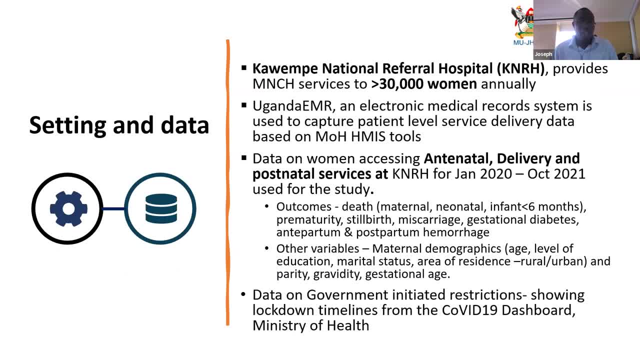 The system is based on the means of health management information system tools And, in particular, we use data for the period January 2020 to October 2021.. Wow, That's very interesting. I'm curious to see your findings for our study. 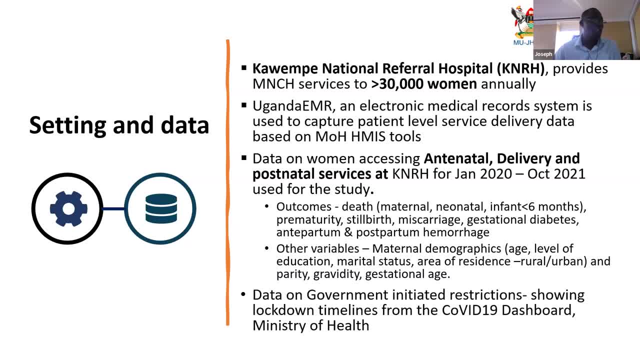 The specific outcomes for our study are death, neonatal maternal death, neonatal death and infant. Infant is just six months. That's just an aesthetic institution. Prematurity, stillbirths, miscarriage, gestational diabetes, at-partum and postpartum human rage. 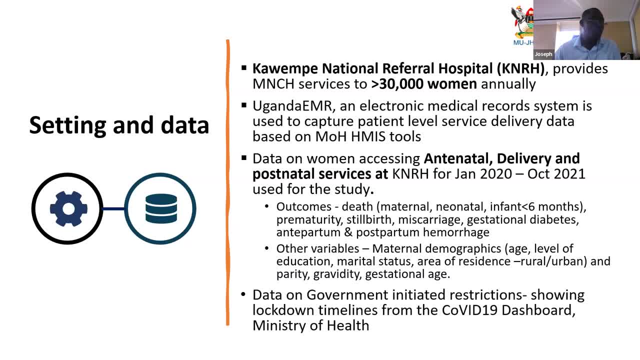 The variables that we extracted and included in our data include maternal demographics, such as age, level of education, myofascial disease status, areas of residence, and also we have data on particular ability and recession age. We also extracted data from the Minnesota Health COVID-19 Dashboard, which had information 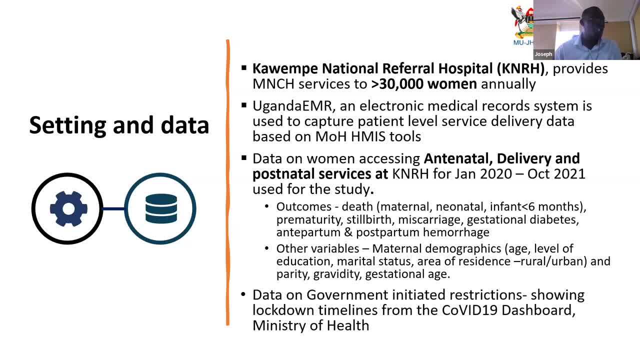 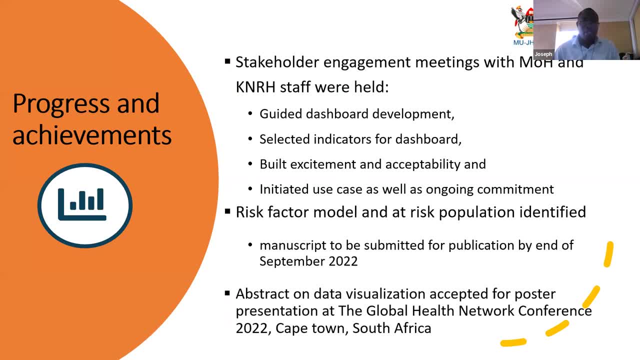 on the time, the lockdown timelines that were initiated by the government. So, in terms of progress and achievements, some of this is that we have stakeholder engagement meetings with Minnesota Health and Kawepe National Hospital staff. The meetings are particularly intended to get guidance on dashboard development selection. 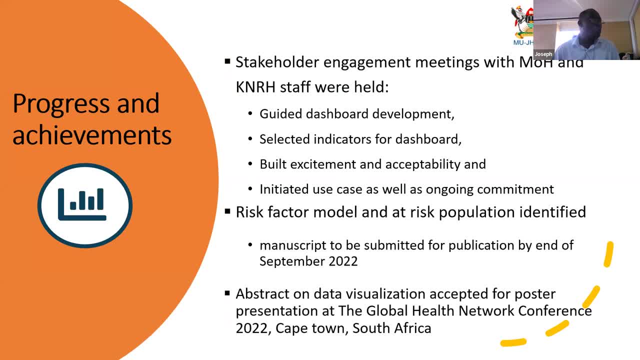 of indicators to be included in the dashboard, but also we wanted to build excitement and acceptability among these key stakeholders and initiate a use case as well as ongoing commitment from this particular group of people, because they were the ones that needed that engagement To benefit from this dashboard. 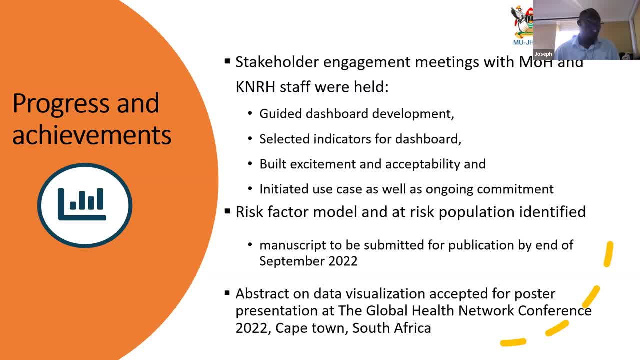 We also intended to develop the risk factor model, which we did and achieved that. The manuscript of this is intended to be submitted by publication by the end of September. We also developed an abstract from data visualization. This has been recorded for poster presentation at the Global Health Network Conference in. 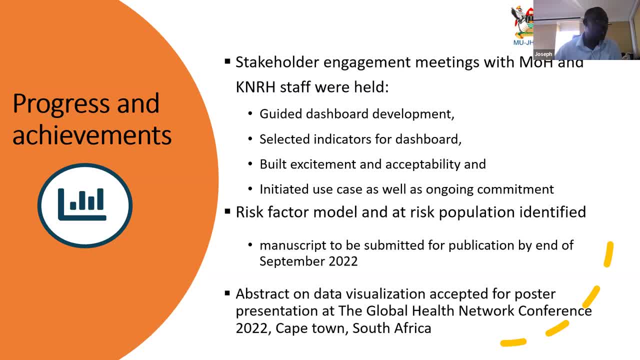 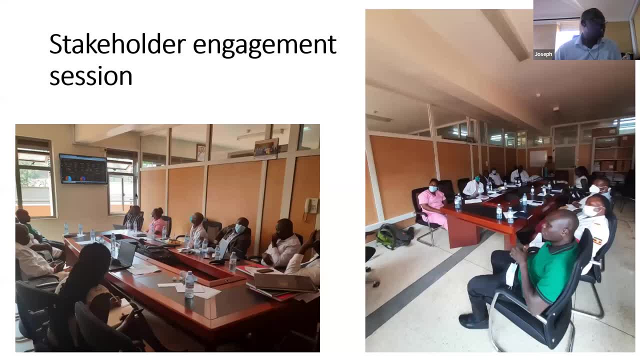 Cape Town, South Africa. It's due this November 2022.. Just to show you our stakeholders in one of the engagement meetings: On the left there, you can see the dashboard on the screen being reviewed and members are giving feedback on what it looks like and how it can be helpful to them. 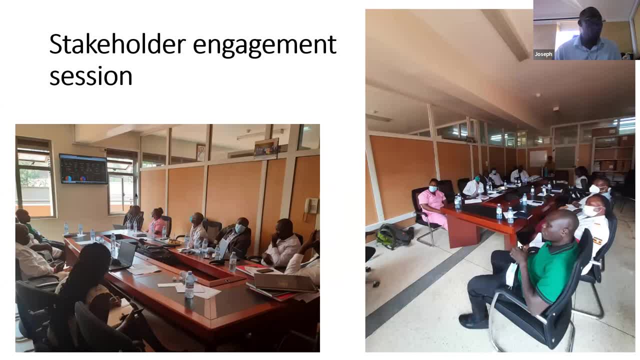 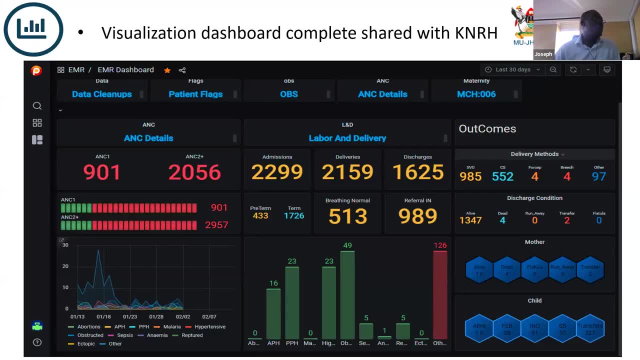 And the same thing on the right, looking at the dashboard hidden from our view here. So this is just the dashboard. The more clearer view, the kind of indicators that will be that's shown on the dashboard will have information on continental labor and delivery and specific outcomes. 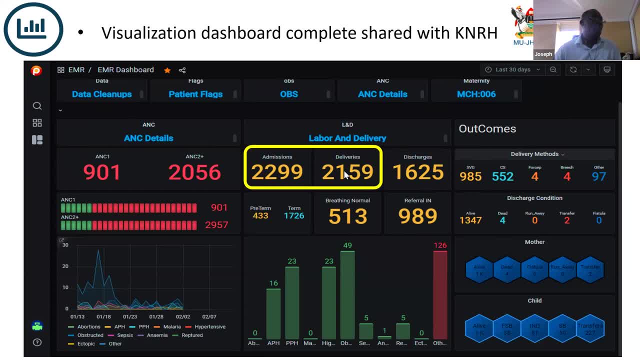 So in particular for this period. So the dashboard can be customized. The user can extract data for a day, a week, a month or a quarter and therefore these statistics will represent the period that the user selects. So, for example, here there were 2000,. we have over 2000 admissions and then we had 2159. 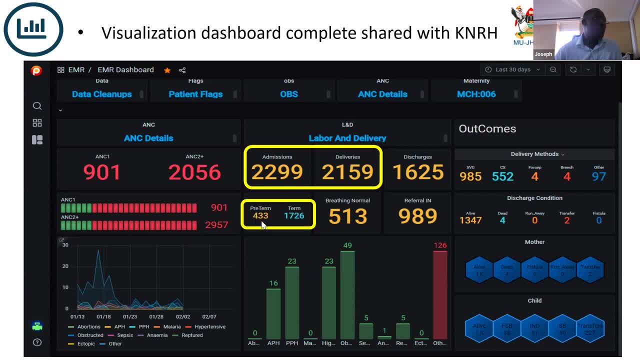 deliveries. Out of those deliveries, we see that 434 are preterm, whereas 10 were 1726.. The same dashboard could show the other outcomes that we've just mentioned earlier, and this is what is would help the hospital management, help their providers, to make broad decisions. 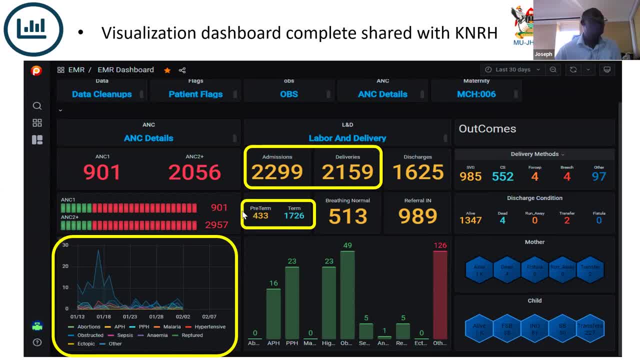 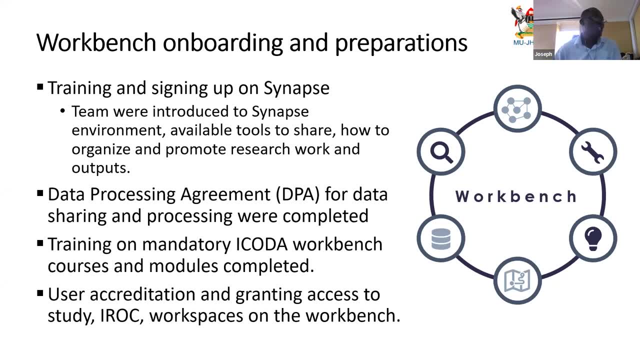 about service delivery in the hospital. So, in terms of the workbench, onboarding and preparation, our team were really naive about signups, So we had training on signing up for signups which introduced the team to the environment and the team was shown available tools: available tools to share, to organize and promote. 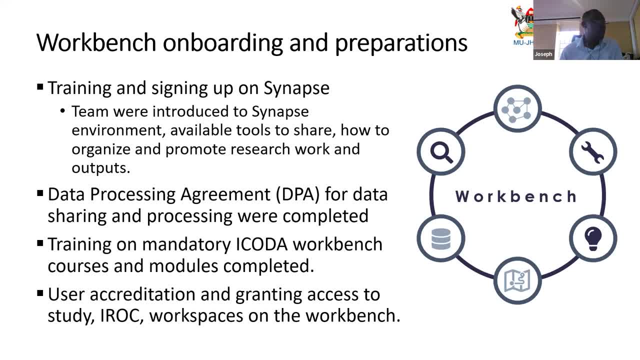 research within the environment. We did sign up to data processing department and for further training on the mandatory workbench courses and modules. and, finally, the team members were accredited for related practices through the study work ILOPS- study works based on the work page. 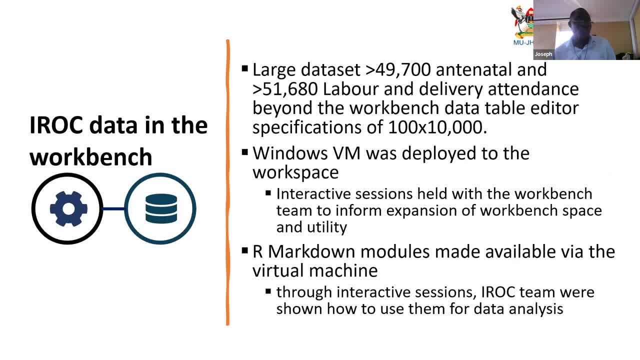 One of our experiences- our data in the work page- is that we have quite a large data set, as you've seen in the dashboard. Particularly for this study, we had extracted over 49,000 antenatal records and over 51,000 labour and delivery records, and this, however. 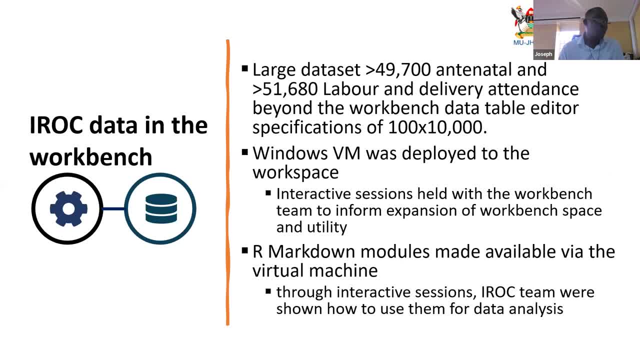 we noted were beyond the work page data editor specifications that had 110,000 records. So therefore a Windows VM was deployed for the workspace and we had interactive sessions with the work page team to inform these sessions particularly, And that's also to understand the work page space and 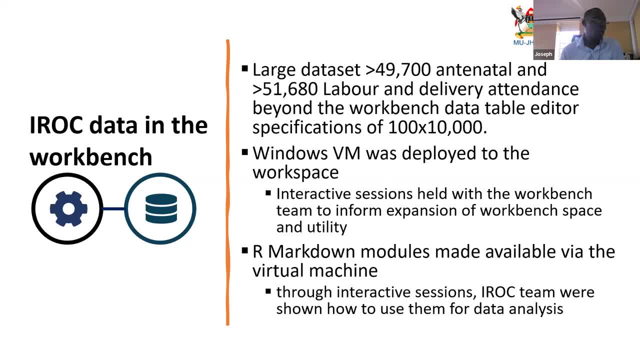 utility and further interactions while I use this interaction was also useful for the team to understand the need of the different users in the work page. Given our huge data sets, the team and given that we had deployed the Windows VM, the team was able to extract. 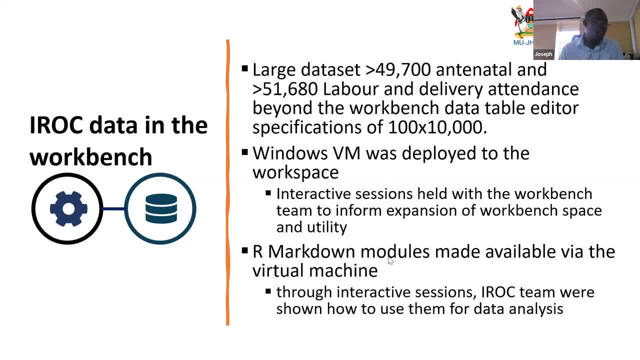 the Aura Markdown modules and these were made available in the VM machine and we also had further interaction with the work page team. We also had further interaction with the work page team. We also had further interaction with the work page team. We also had interactive sessions where the team- our team- was shown how to use the modules for data analysis. 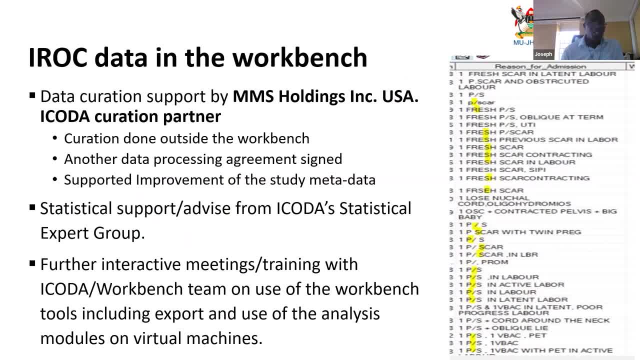 Just before our data was uploaded onto the work page, we had data curation, which was supported by MMS Holdings Inc. and just to our right- you can see the kind of data that we are talking about- to the group curation board. So this curation cost was a huge dataset. 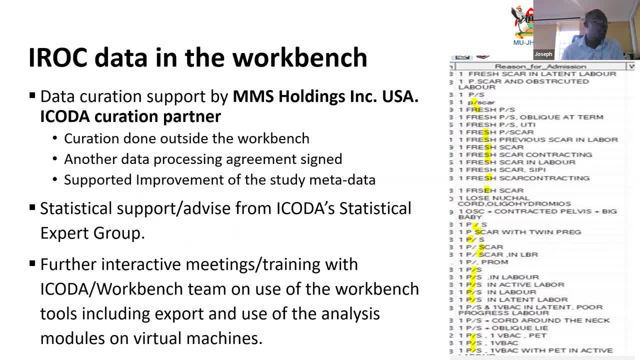 Recognition was requested to be done outside the workbench. Therefore, we had to sign another data processing agreement with MMS Holdings Inc. and the team also helped us to improve our study metadata. We also got additional support from the student expert group and a lot of further interaction meetings. training with the WorkPage team helped us to. 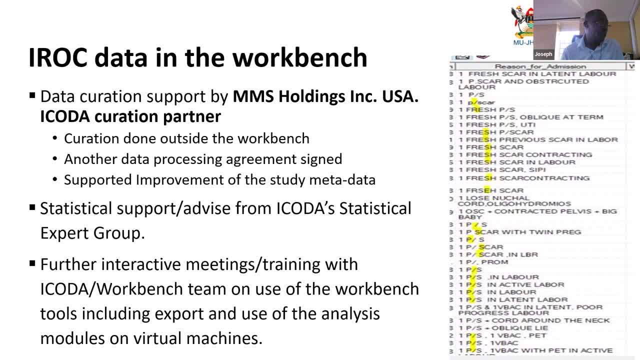 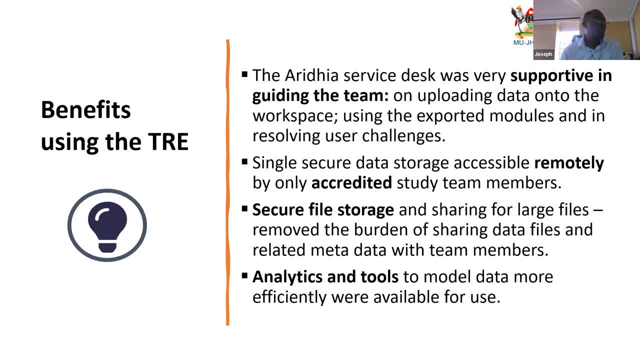 really understand how to use the WorkPage for our analysis of the virtual machine, Our benefits that we realized. we thought that the WorkPage team was very supportive in guiding our team all through the process, uploading our data onto our space, using the exported modules, and in resolving any other challenges that were. 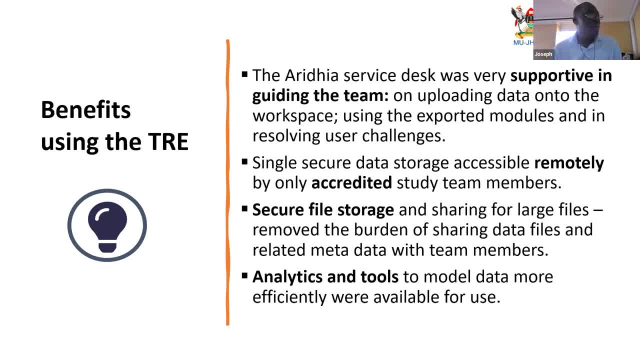 arising as we were working through the WorkPage. We noted that our data was in a single space, single secure data space, and only accredited study team members were able to access this data. There was also secure file storage and sharing of large files was removed As opposed to other. 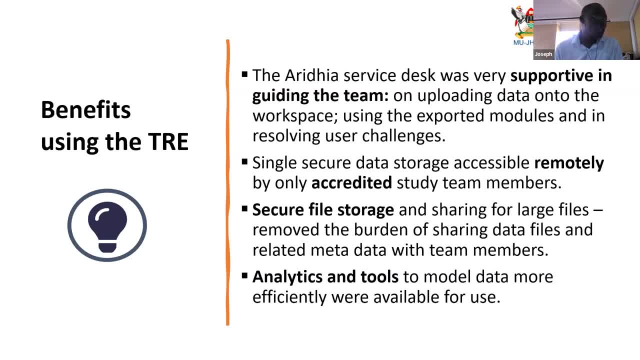 cases where files would be shared among co-users, all the members were able to go into the WorkPage at any one time and be able to do what we had to do within our project. The analytics and tools to model our data were very efficient and available for use whenever we wanted to. 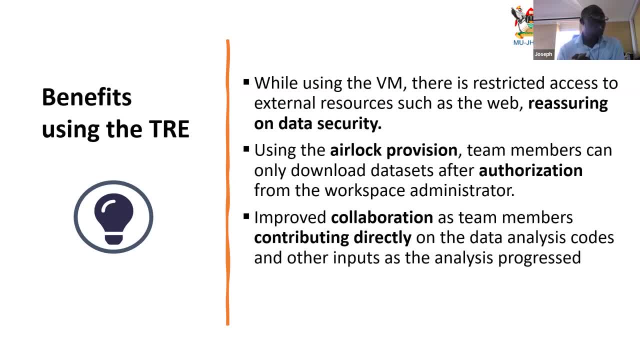 While using the VM, we also noted restrictions. We had limited access to external sources such as the web- and this was reassuring in our data security- And also using the dialog provision available in the WorkPage. the team members could only download datasets after authorization from the workspace administrator. And again, 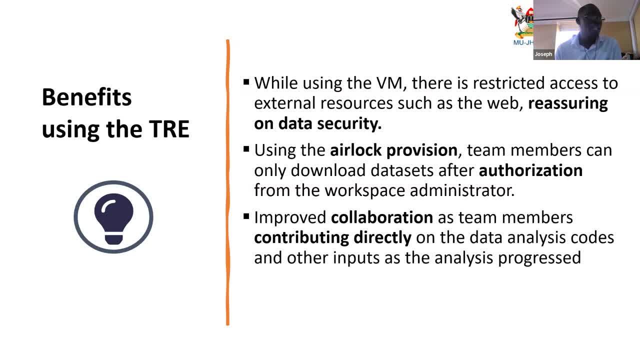 this was really reassuring in security of our data and how the data could be shared around. We thought that there was input collaboration among the members, as members were able to contribute directly onto the data analysis code and other inputs as the analysis progressed. Just a bit of challenges, but we think. 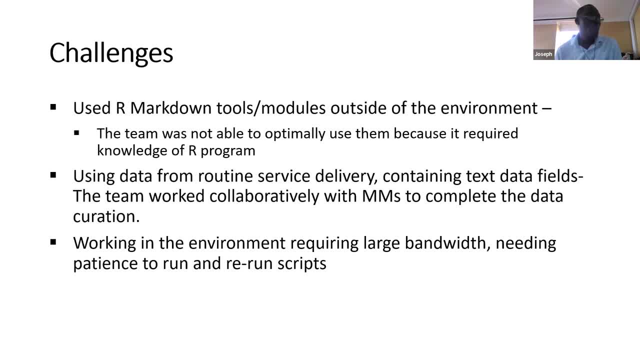 that these were resolved as we went along with the work. So these are not challenges that failed us completely, but were resolved within the period that we were doing the WorkPage. There are markdown and feedback that are still going on in the work. The support staff included a lot of. 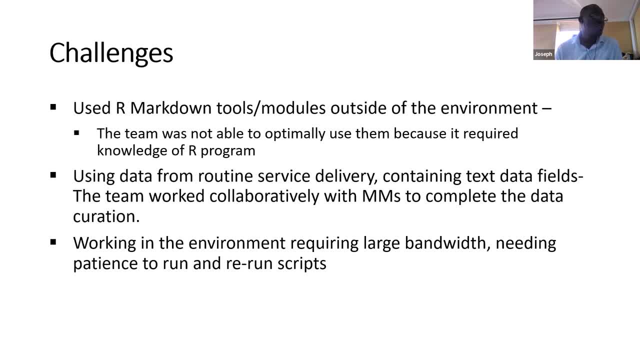 work, and this is because using them outside the environment needed us or team members to have some idea of using the R program, which to some was quite new and that was a bit challenging, but we were able to overcome that. Our data being routined is then limbs data And, as you've seen, having a lot of text data fields working collaboratively with our team members, but we also have some capabilities within the data analysis program. there were no events like this, So we also did some planning to automate this and해주 a lot of work and support projects during this time, when we were able to meet a lot of these targets. So these are some issues related to data analysis and investment. 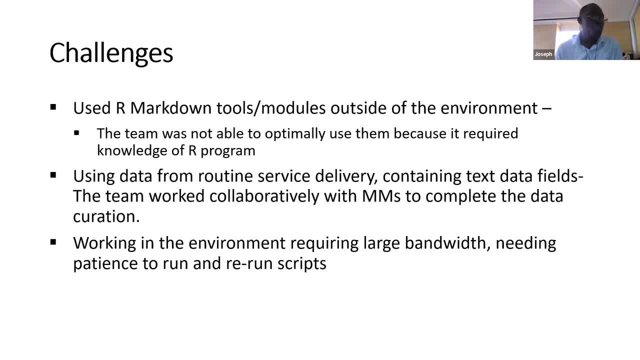 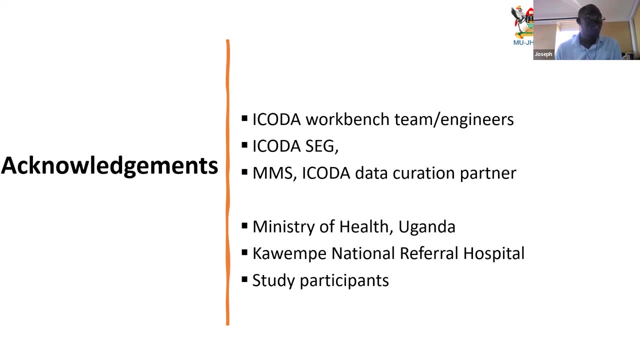 the mms team were able to complete the data curation and also, working in the environment, required large bandwidth and needing some patients to run and rerun our scripts. just to acknowledge the team that really worked tirelessly with us: the workbench team and engineers, the statsco expert group, the mms- i called the data curation partner. means of health. 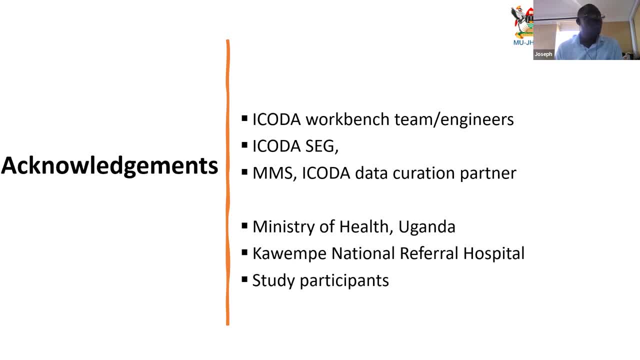 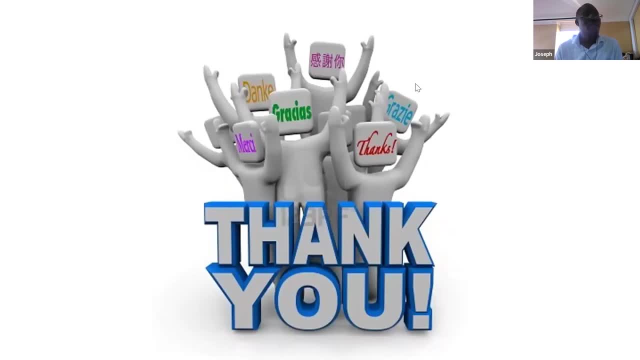 omp national repair hospital and the study participant whose data was used for this project. thank you very much. that's brilliant. thank you, joseph. really, really interesting and inspiring. um, let's um. if you could stop sharing, let's pass the baton to carl, who can take us through um how his team have been using. 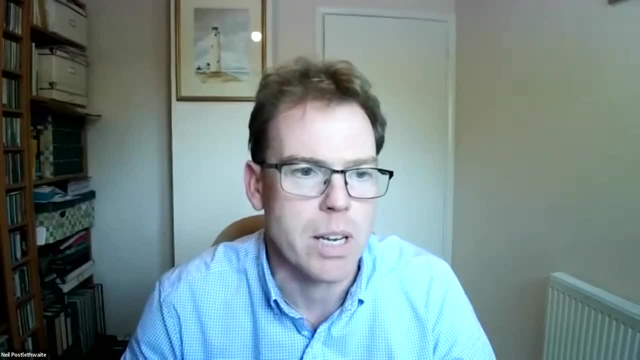 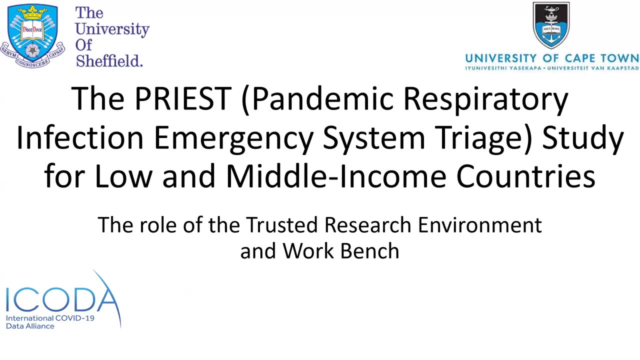 the mms team and the mms team have been using the mms team and the mms team have been using the tiaris, and then we can open up for questions and q a. so, carl, over to you. okay, i hope you can see my presentation. um, so, i'm carl rickwitz. i'm the principal investigator. 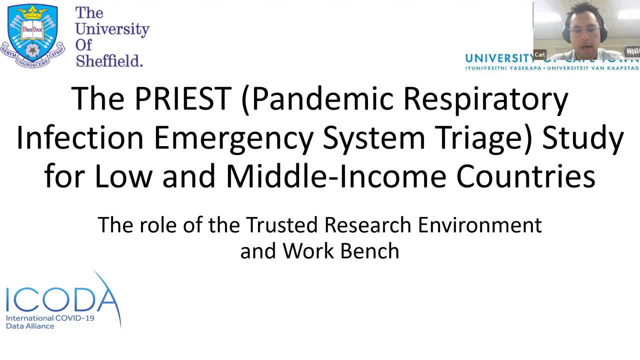 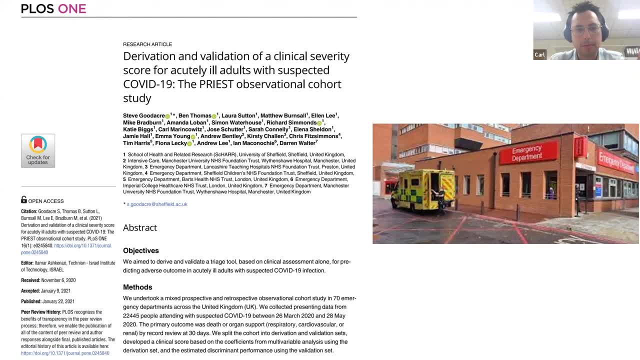 for the priest in lower middle income studies and what this is based on is about two years ago now in the uk, we had just completed a large cohort study where we collected data on own over 40 emergency departments in the uk in order to develop a triage tool which could be used to 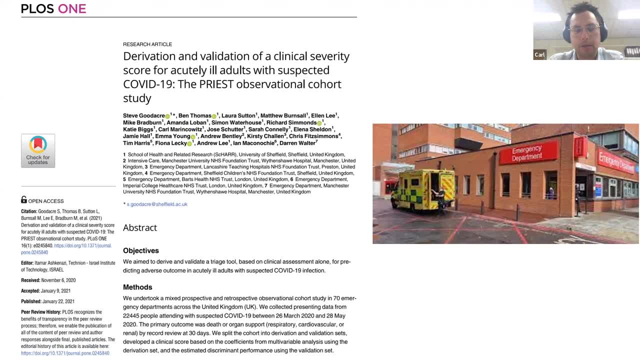 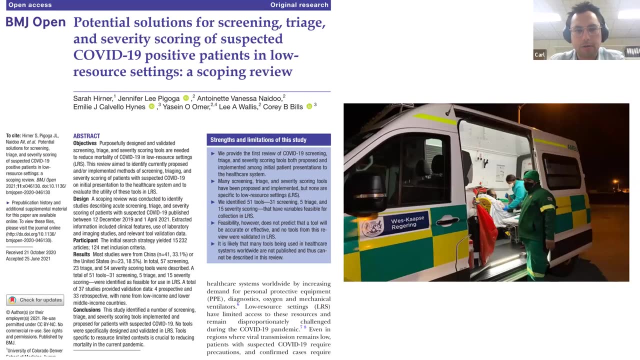 rapidly and transparently determine if patients were suspected covered needed inpatient hospital admission from the emergency department, based on their risk of subsequent deterioration. shortly after this, our colleagues and collaborators at the university of cape town looked at the literature and found that, although there were lots of triage tools, 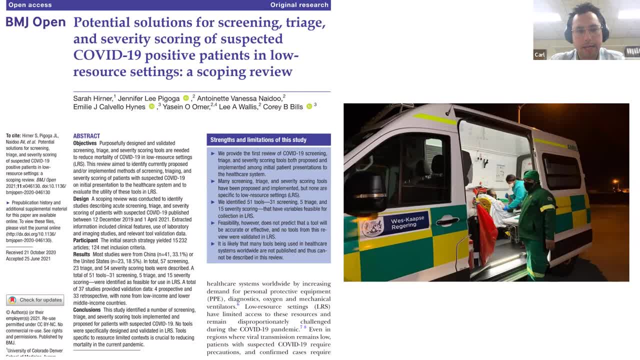 being developed in high-income settings that there wasn't really a need to be any tools which should be validated or developed in lower income, low or middle income settings. and this was a bit of a problem for our colleagues in the western cape, as they weren't sure things like the priest tool were applicable there. so on the basis of this, we 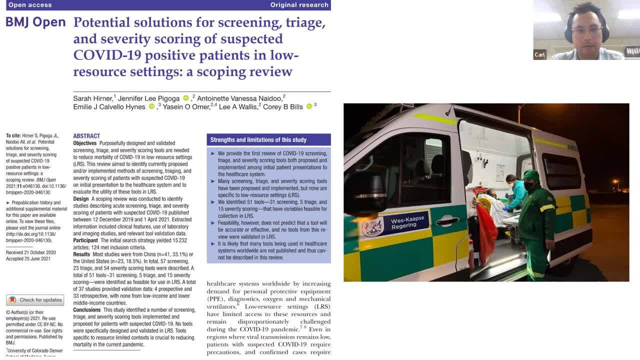 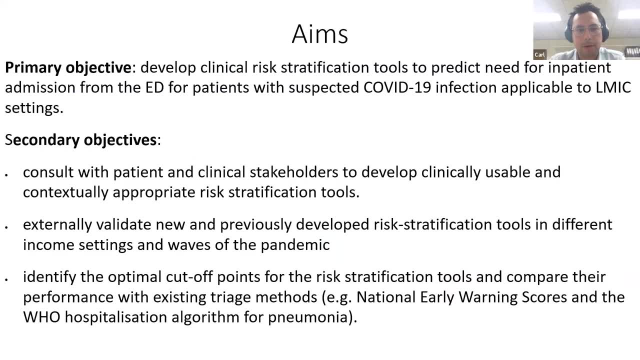 developed a collaboration of partnership and applied for the icoda funding as part of a pilot project, and what we aim to do is essentially develop a priest-like risk stratification clinical tool which could be used to help triage patients with suspected covered in emergency departments and lower middle income settings, specifically the 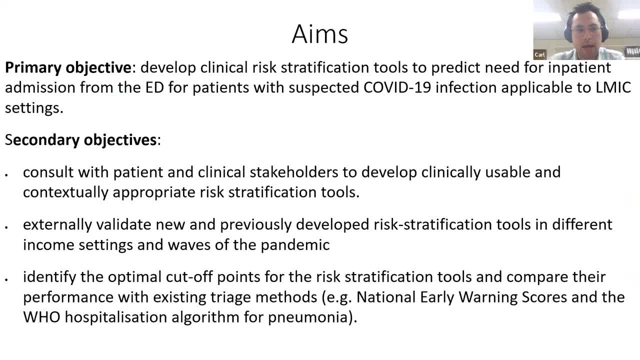 western cape and also sedan, and key to that is involvement in clinical and patient stakeholders to make sure that the triage tools are acceptable both to patients and clinicians and are also usable, and we also explored the use of machine learning techniques to see if prediction could be improved. 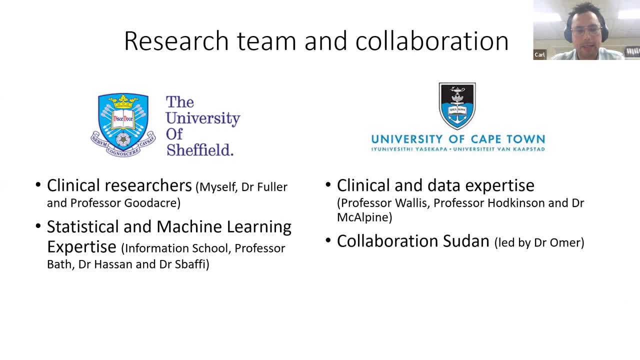 so in terms of our team what we've had is research. the university of sheffield had been involved in the original pre-study in the uk and that was the basis kind of for our machine learning and other modeling techniques and also for triage tool developed clinically and then from the 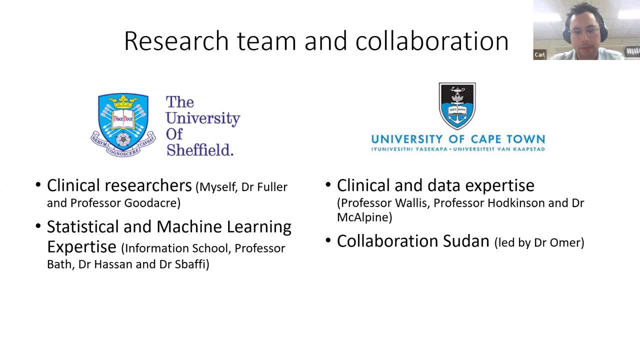 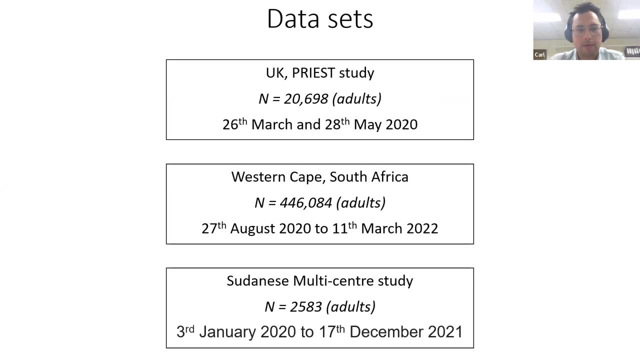 university of cape town. we had clinical expertise from people like professor wallace and also an existing collaboration in sedan. we used three quite large cohorts for our study. so the first is from the uk, which is the uk pre-study, with around 20 000 patients from the first wave. 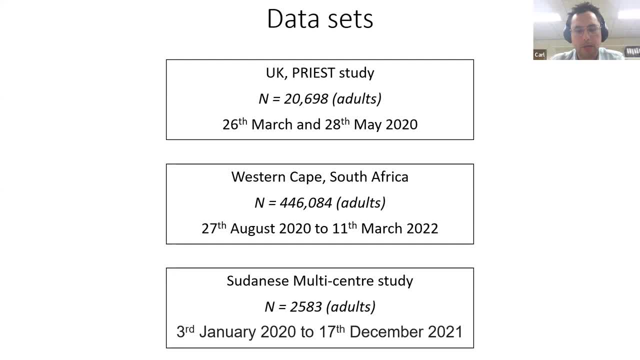 who had presented with suspected coverage and that had been used to develop the original priest tool. luckily, in the western cape, shortly before the outbreak of covert, that implemented electronic records, so we were able to suck out huge amounts of data and about 450 adults who presented from august 2020 to march 2022 with suspected coverage. 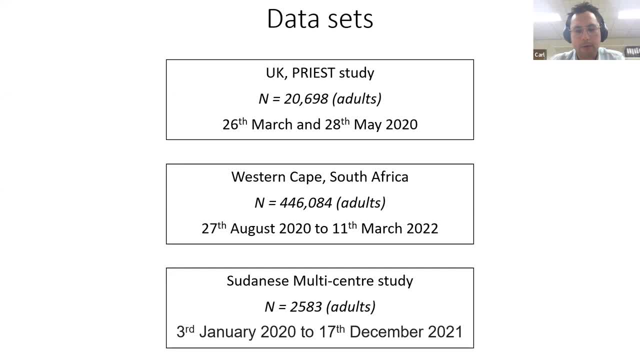 and then, finally, we had an ongoing multi-center cohort study with the university of cape town, which is a cohort study that was conducted in the west, in cape and from sedan, from an existing collaboration with the university of cape town, there was also an ongoing multi-center cohort. 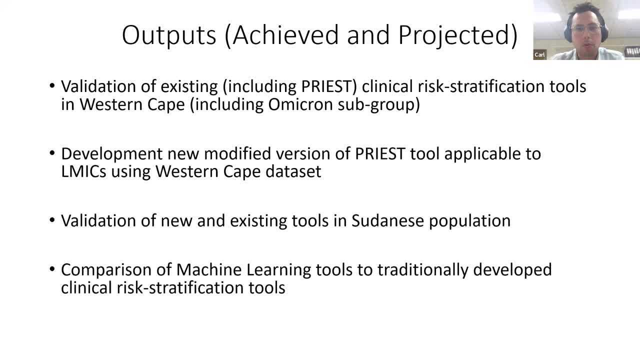 study collecting data from patients with suspected cohort, presenting to four senses in um sedan, basically the cartoon region. so what we're aiming to achieve from this we've already achieved: about to determine the need for inpatient admission, and that includes the original pre-stool as well as. 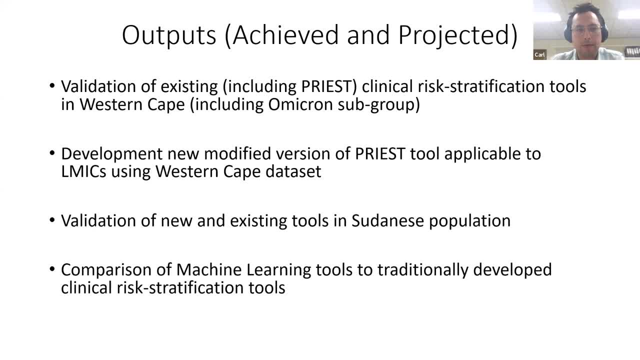 things like NEWS2, which were routinely used in the UK. We've developed a new modified version of the pre-stool using Western Cape data, which is applicable for use in South Africa and other settings which use similar triage methods in the emergency department, and we're also validating. 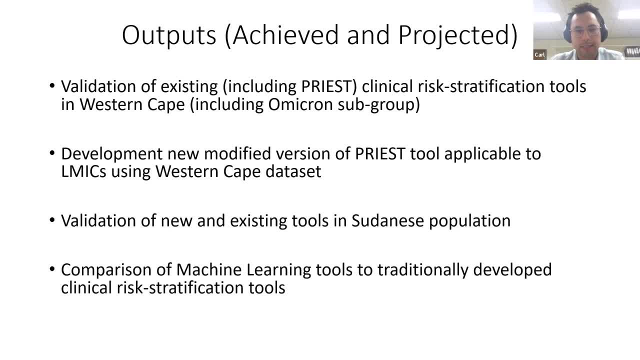 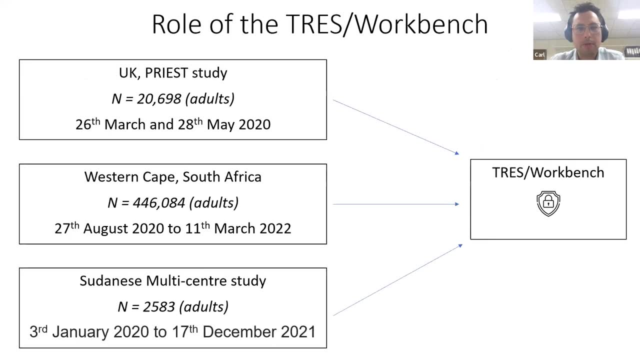 the new tool and other existing tools in the Sudanese cohort study We've also done some machine learning to see if it can improve prediction of adverse outcomes and therefore need for inpatient admission. So in terms of the role that the trusted research environment has played, the main one is for us has been a central, secure repository in which we can keep. 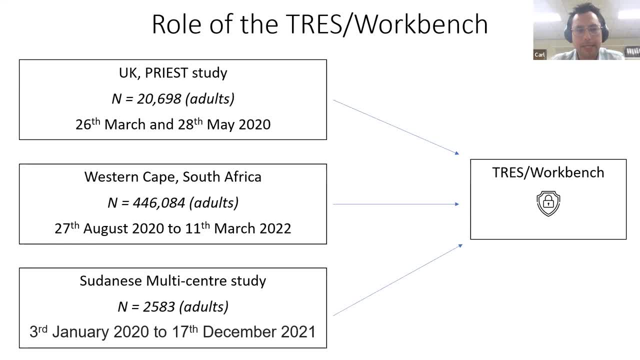 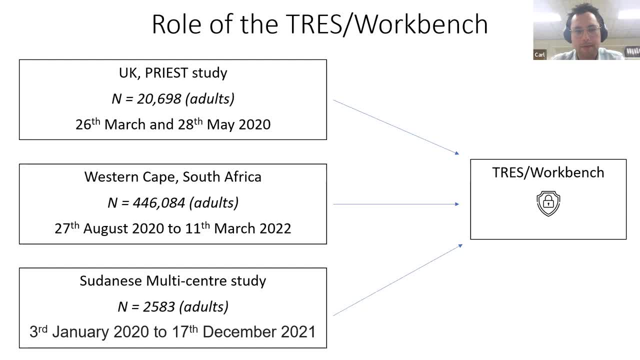 We've been able to do that. So we've been able to do that. We've got specific data sharing agreements attached to it and that means that they have to be processed and used and shared in certain ways, and the trusted research environment has meant that there's a central repository where the 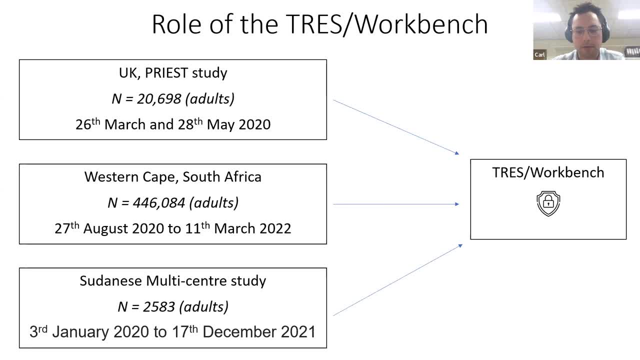 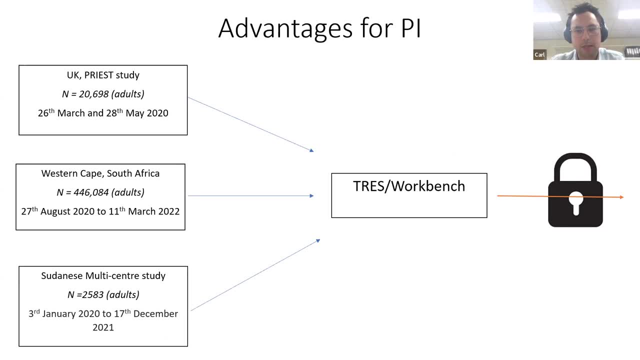 international team can access and keep all that data in a secure way. From my perspective as a PI, it's meant that I've had control of those data sets and have ensured that any data flow from the trusted research environment to members of the research team has been in accordance. 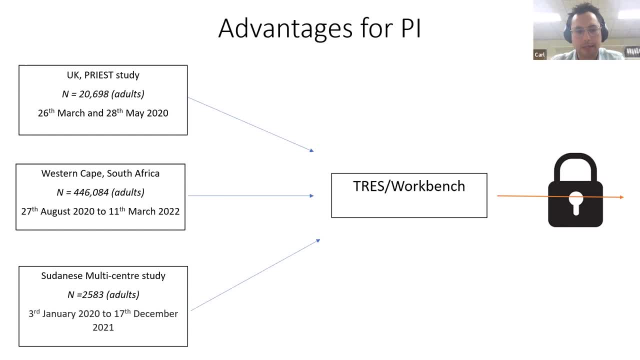 with the data sharing agreements and stipulations of the data controllers, and there are three essential data controllers. so one is the University of Sheffield for the UK priest data, for the Western Cape data it's the Ministry of Health in the Western Cape, and from Sudan it's 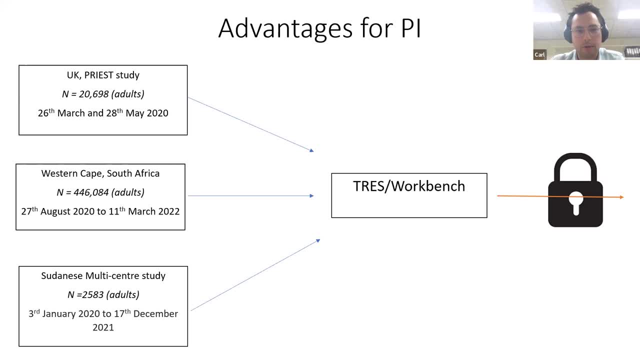 the Ministry of Health from Sudan. there are various rules which govern how we can share and access that data, and I've been able to keep an overview, as a PI, that we're sharing the data in a way which fulfills our data sharing agreements and obligations to the data controllers. 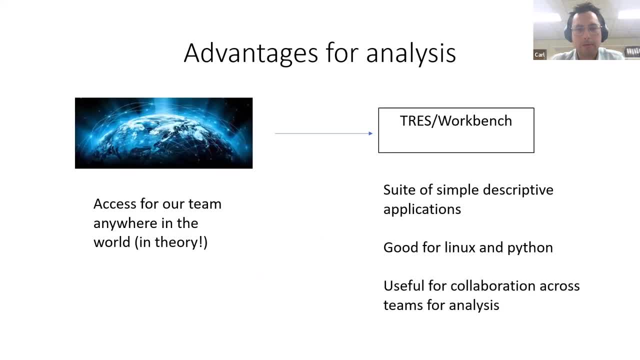 in terms of analysis. I mean the main advantage is that you can access the trusted research environment and the virtual machines which we've been using in theory from anywhere in the world, and that's been pretty convenient for our team. the simple suite of descriptive applications which would be made available on the workbench are pretty good for simple descriptive statistics. 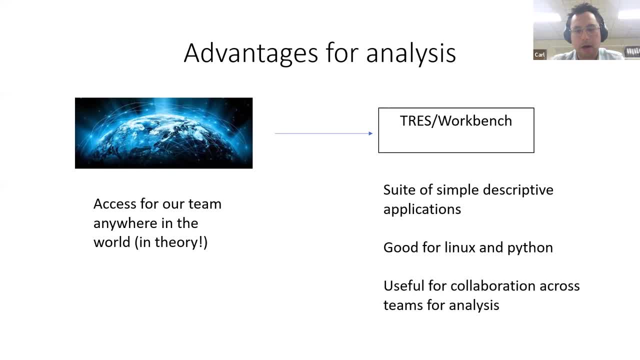 comparison of the data sets, and it's meant that we've been able to compile comparisons of the different population characteristics relatively easily in order to inform a more complex analysis. for our analysis analysts, which use Linux and Python, it's set up for that, and Medina, who's the 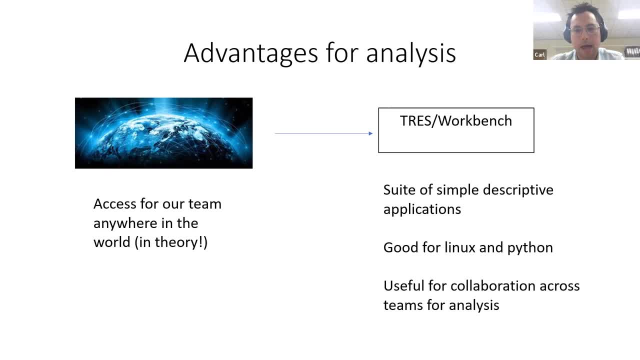 main analyst working on it has found it very good for that and, although it's been less of an issue for us because most of the analysis has been done by the University of Sheffield team, it is a very useful function if you've got analysts based different parts of the world or not on the 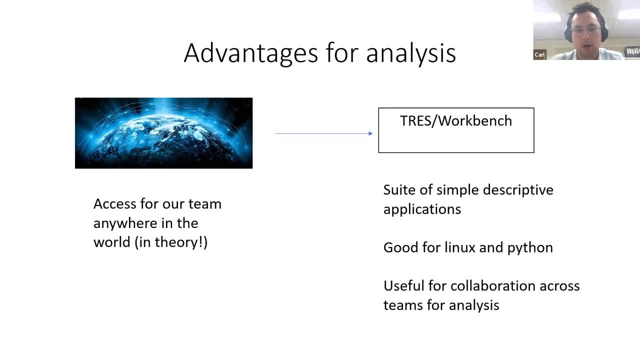 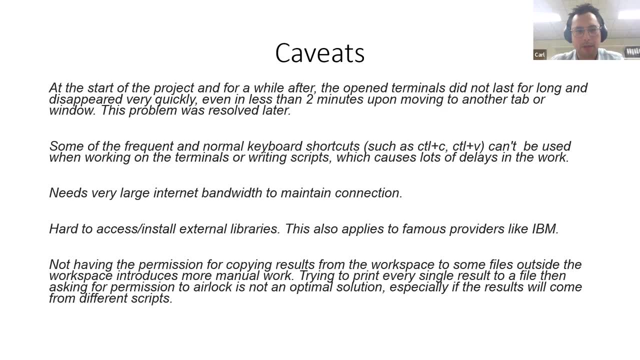 same geographical location, as they can all work simultaneously on the data sets and share code and things like that. however, there have been a few issues, so these are. I asked everyone who's part of the analysis team to fill in a quick survey about how they're found using the trusted research. 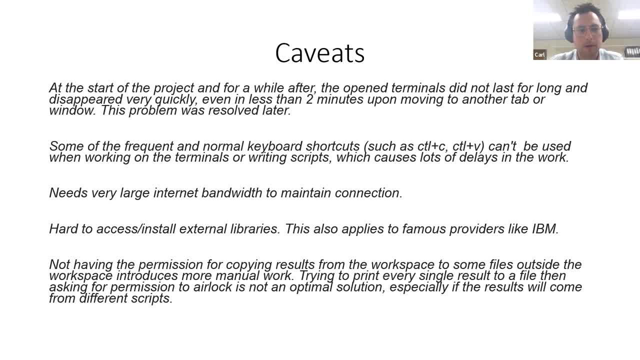 environment, and this is the kind of feedback which I got back. so one of the things is that you do need large bandwidth to maintain the connection and that can cut out and that can sometimes lead to lots of analysis and data because of the way that the trusted research environment is set up in such 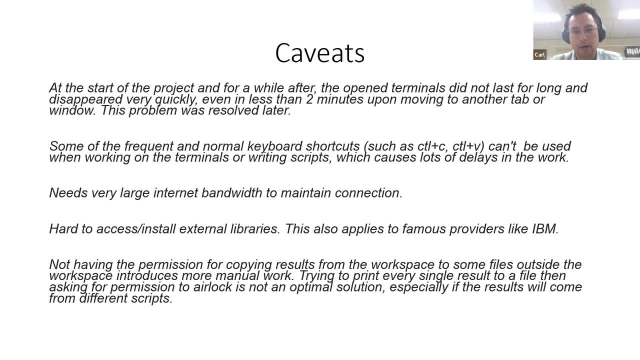 a secure way. it's not got direct access to the internet, it's very hard to import scripts and things or copy and paste or to upload extensions to things like R or Python. also, there is limited ability to upload things like Stata or SPSS, which we did persevere with, and although 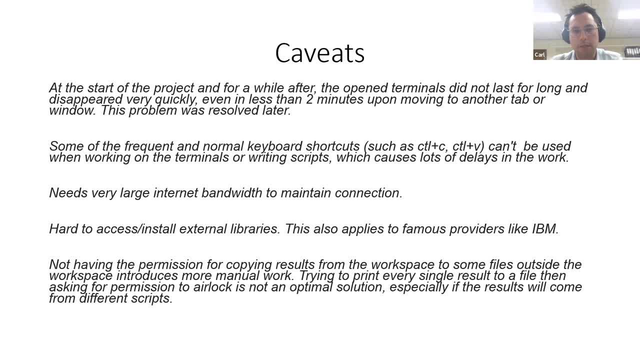 some of the analysis has been solely done on the trusted research environment workbench, particularly with the Sudanese data, because of the nature of the data sharing agreement. other bits of analysis we've taken off in accordance with the stipulations of the data sharing agreements and analyzed within the University of Sheffield. so I think the main advantages of the workbench- 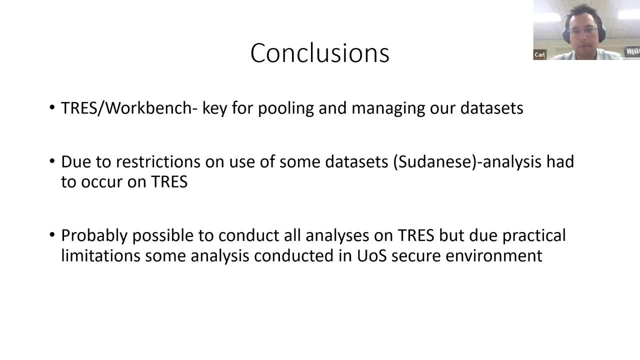 trusted research environment for us, have been pooling and managing our data sets, especially across the kind of global team that we have, so we've been able to keep them in a secure place. there's not been sending data sets, you know, by email or things like that. we've been able to. 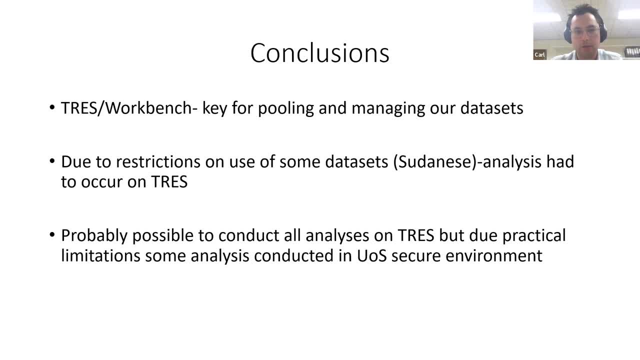 upload them all to the trusted research environment and keep them there, and it's a central repository similar to like a shared drive that we'd normally routinely use in the University of Sheffield, but on an international scale. due to the restrictions of the data sharing agreements, some of the analysis we've had to 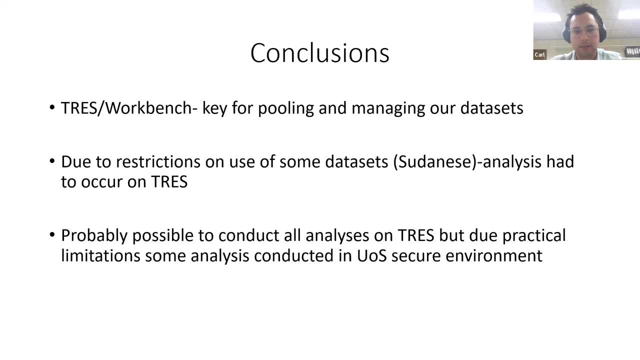 solely do on the trusted research environment and that is, you know, very feasible, especially if you're a Python user or using applications which are already available. but there are, you know, some issues with ease and practicality of analysis and, for us, some of the analysis we've 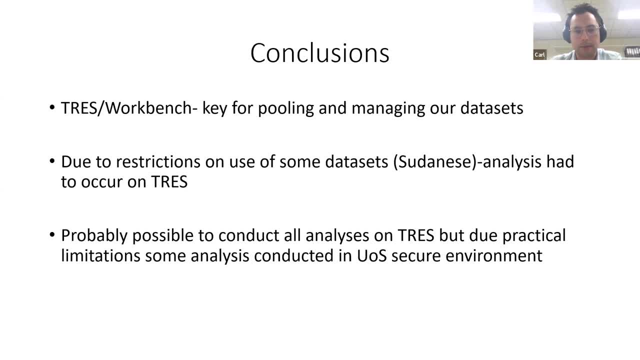 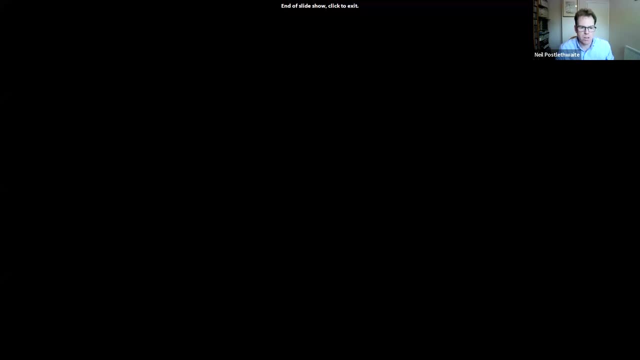 done off the trusted research environment within the University of Sheffield just because it's been easier for us. thank you, brilliant. thanks, Carl, really insightful. yeah, if you stop sharing, that would be good, let me. let me just pick up. that was. that was really interesting and and thank you to you both. 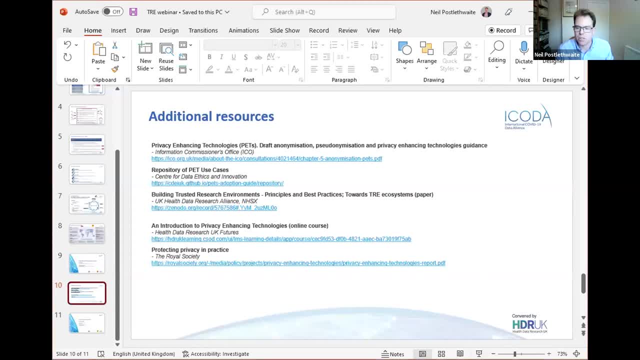 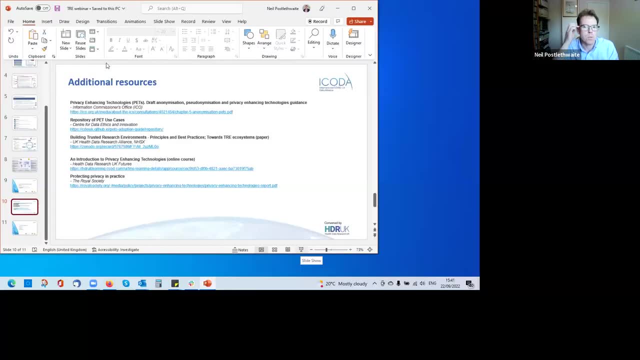 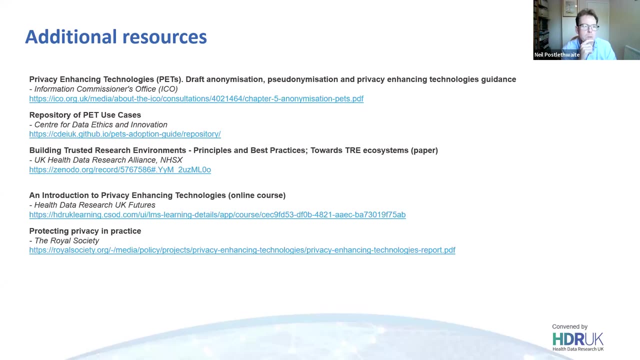 for for sharing very openly the the pros and the cons here, as, as we work with some of these emerging technologies, a set of resources that we've just put together with you, so we will share the presentation um in uh in a pdf afterwards. so a couple of things that you might want to look at in terms of more. 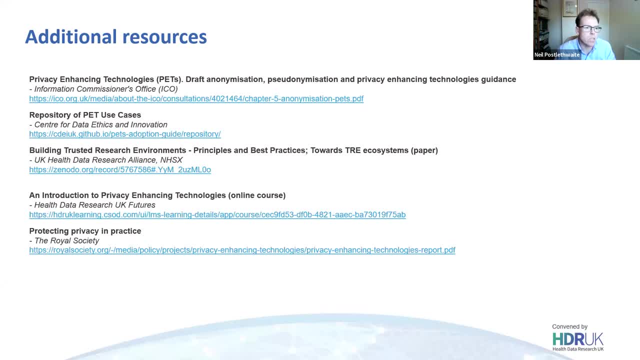 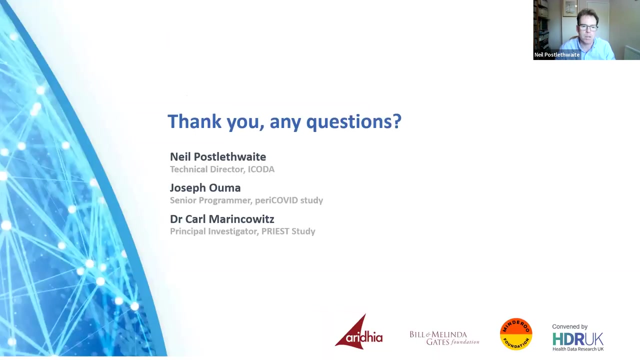 information on privacy enhancing technologies, um, trusted research environments and some online courses and and protecting privacy in practice- some really interesting researches and reset resources, if i could speak um in a rapidly moving area and uh, yes, so with that um, I'm gonna move us across into the Q&A. so, Joseph and Carl, if you'd like to come back, 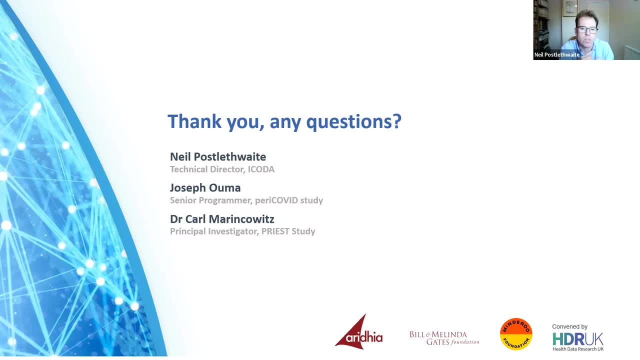 on camera. let's see what questions that we've got um. hopefully, that will then result in not just people seeing me, but they'll see the three of us um the first question I'll answer, which is: can the slides be shared? um? yes, Dorothy, absolutely we will. um share a pdf copy of the powerpoint and also support and contact you by using pdf to share all this information for up there in some of the setting, especially about any data that you might want. your surf—ование will not be able to make you know nodes. —V온, are you? just, you have pero昭 and I ran that question into that. but you can see that's a 와. 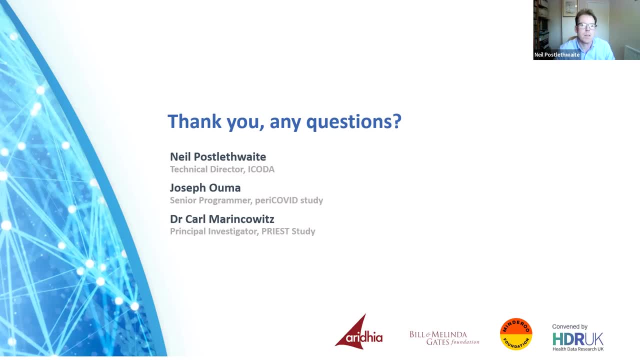 dVm Gonzalo, that's выше, whose baptist hope we have. you're wieder, delie. Benedict Jahres Markus session is being recorded, so the recording will be made available, so hopefully that is useful. um. the first question I can see um is, uh, from Edel McNamara. in general, do you think there's a move? 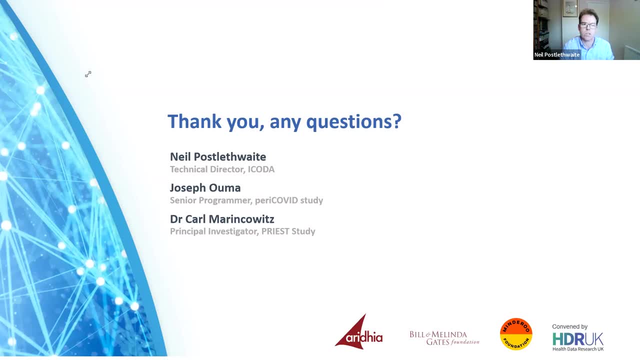 towards the use of privacy enhancing Technologies, such as trusted research environments within research, as opposed to methods like sending data directly between individuals and institutions. um, so let me start with Carl and then I'll pass to Joseph, just for thoughts on that. so, use of TREs as opposed to sending data directly between individuals and institutions. Carl, what are your? 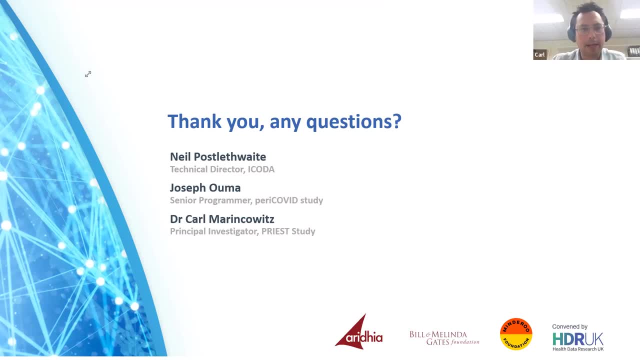 thoughts. I mean I can only talk from the UK experience, but for things like NHS digital, um, there definitely is this move and I think the Welsh sale system is a trusted research environment which is very well established where people are given remote logins to do their analysis on NHS digital, which is NHS data. 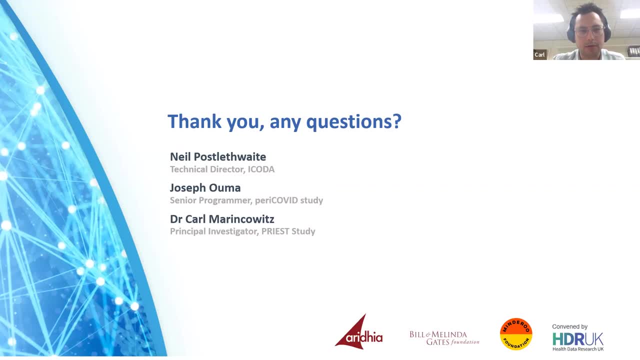 um, as opposed to sending out chunks of data which they then kind of lose control over. the very, because the data sharing group is associated with them, are very strict. it's very easy to accidentally breach the stipulations. yeah, makes complete sense, Joseph. what, what about you? do you? 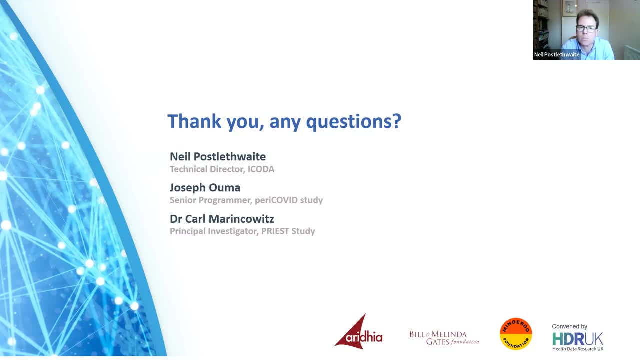 do you see a move towards this from from your perspective? yeah, yeah, I agree, um, because of the, the advantages that we see here and and um, thinking about data security and all the data agreements that we sign- that this becomes a more secure environment to share and work with data. thank you, yeah, thanks, Joseph. 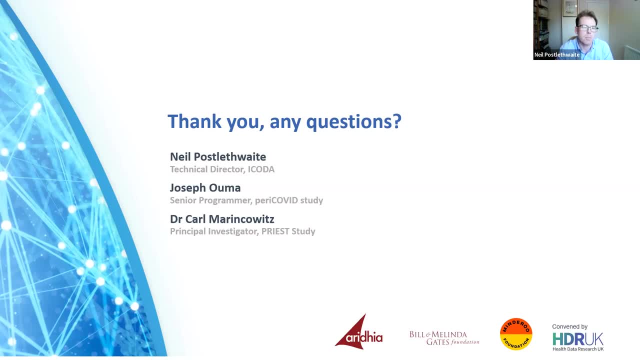 and I would concur with. concur with you both. um you know, the international COVID-19 data Alliance is being joined by Health Data Research UK, who've been a very big proponent over recent years of the use of trusted research environments and, as Carl said, that usage is very widespread within. 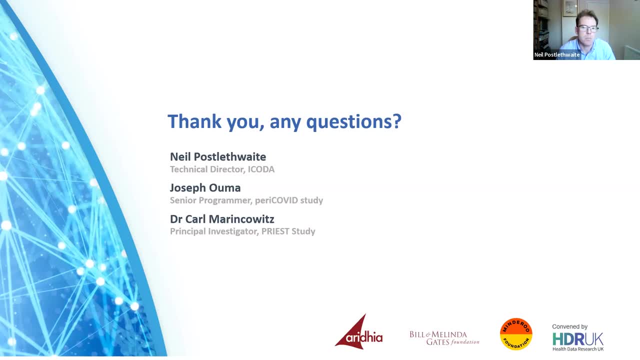 the UK for health data research and- and I think is- is getting a more global spread and, and certainly you know, we've been privileged to welcome the all of the iCoder driver projects to trusted research environments as well. and, as with any new technology, these things will iterate over time and and will 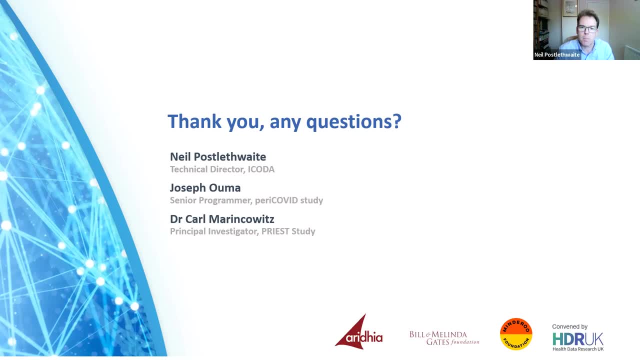 continue to improve. um. next question: um and again- I'll start with Carl and Pastor Joseph- um, what features do you think are missing in trusted research environments? so I think the main issues are kind of ease of analysis I've used not just on this project, I've 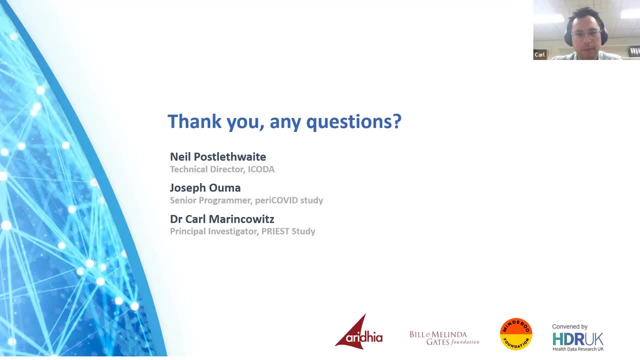 used various types of virtual machines and trusted research environments and there is a kind of a spectrum of how easier it is to applications that you want to use access the internet in a way to download things which are useful, um, and how strict the trusted research environment is and how restricted it isn't doing. 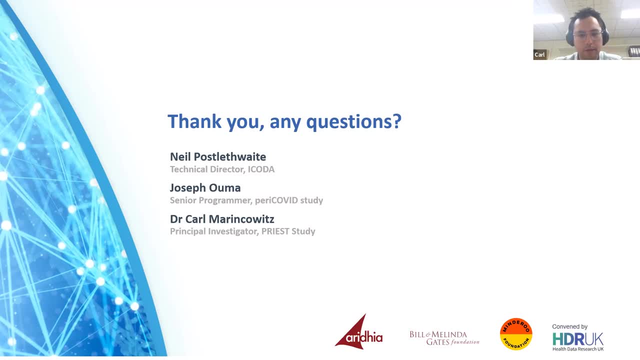 that, and i think what was good with the trusted research environment provided by a coder is some of those default tools which allow you to do simple analysis. um, i think if things develop and those tools get better, then it will um, hopefully reduce need to ask permission to. 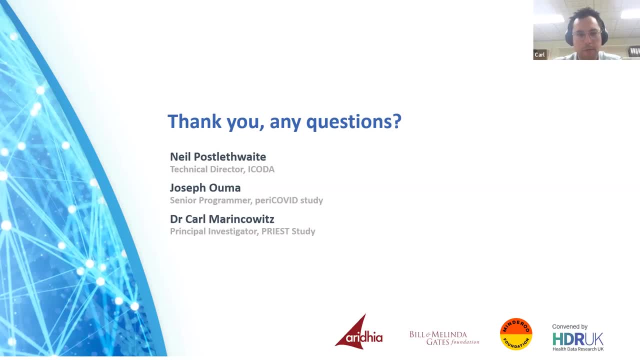 access you know another library or browser stuff to improve the ease of doing the kind of analysis that you want to do? yeah, makes sense, joseph. what about from, from your perspective, anything, anything missing from trusted research environments, at least as you've experienced in this project? yeah, thanks, neil, i think. uh, really similar thoughts. 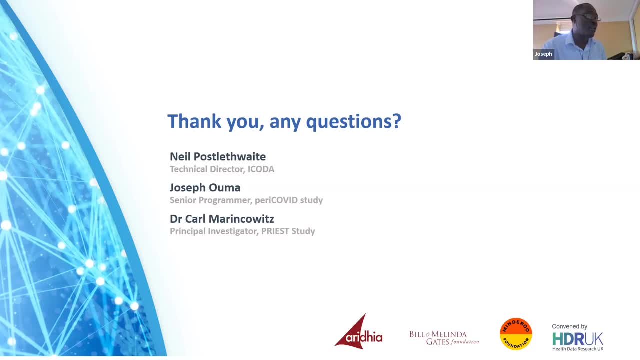 one is the, the tools that you'd like to use, for our case was missing really most of the time, and therefore we had to try and bring this from outside the environment and get to use them there, and then, uh, secondly, i think, uh, the data analysis softwares, for example. this was really in our and. 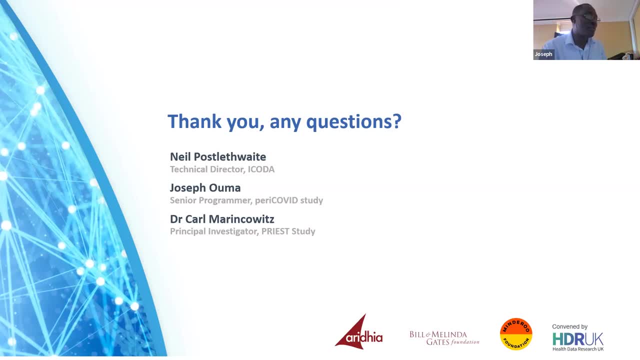 and many and many of our team members were not able to use that initially and we took quite a long, you know, time to get everybody to speed. so, availing more, you know, data analysis software and that analysis tools will be much uh recommended, but also the space, the amount of space available to house. 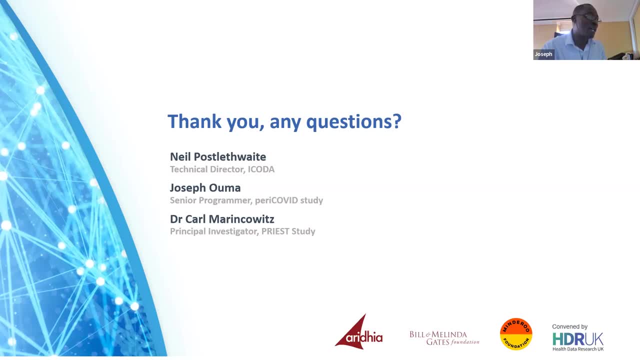 all the data. i think that was kind of holding us back a bit, uh, including a need to have a bigger bandwidth to be able to do what you want to do quite quickly. yeah, so those are my thoughts, really, thank you, thanks, joseph, thanks carl, brilliant um, and i notice also in in the q a um we have. 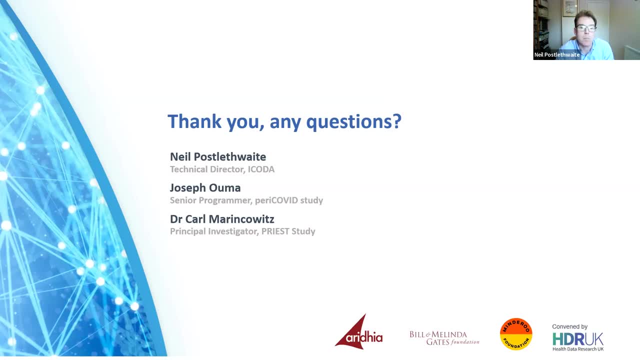 uh, owen, with us from the aridi informatics team who provide our trusted research environment, and he's um indicated that both carl and joseph, he'd love to just have a quick session with both of you to run through some of the the challenges and caveats that you face if you're 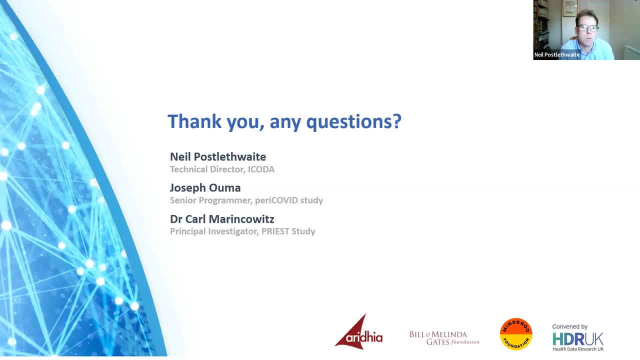 up to up for that. that would be. that would be great and we'll continue to improve the offer here. um slightly different question, not to do, you know, directly with the trusted research environments, but we have a question from james pickett on um any overview of the public and patient involvement. 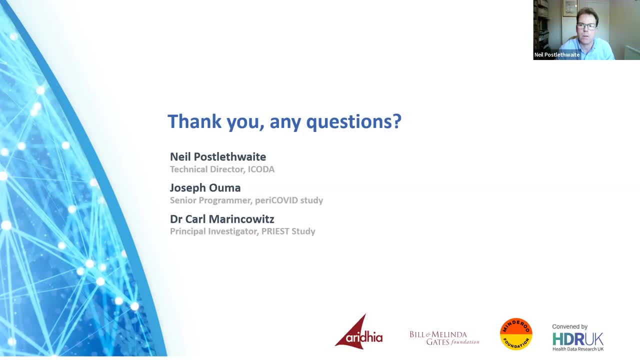 in the project, very interested in joseph's experience um or in sudan in particular. so, joseph, can you give us a a minute or two overview of public and patient and how they were interested, involved in your project? Yeah, thank you Neil and thank you James. 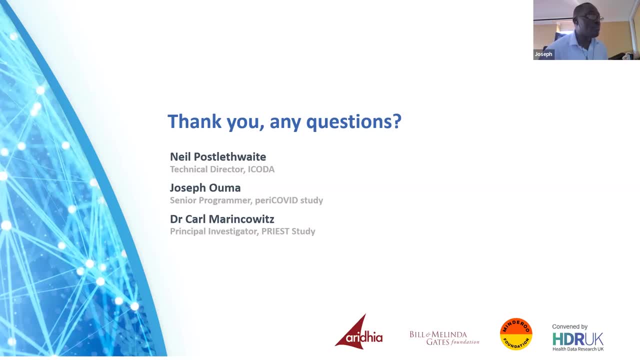 for that question. Yes, our engagement was really more so with the providers, the service providers and the Ministry of Health. So, while we had the engagement workshops to review the data that we are going to use for the dashboard and to review the kind of things that they are interested in, 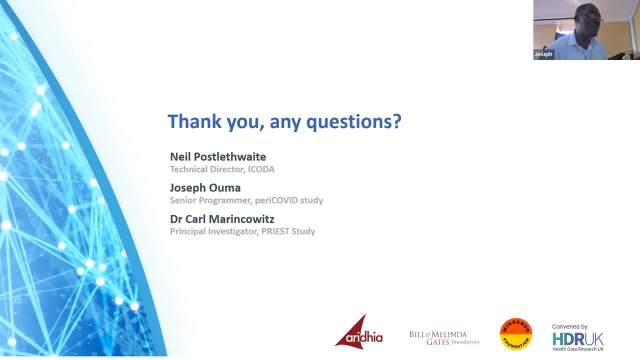 of course, one of the things they were expressing concerns over were the confidentiality of the data and anybody coming within the precincts of the hospital being able to identify and see who is in the data. But I think they quite understood the confidence we had and the confidence we gave them. 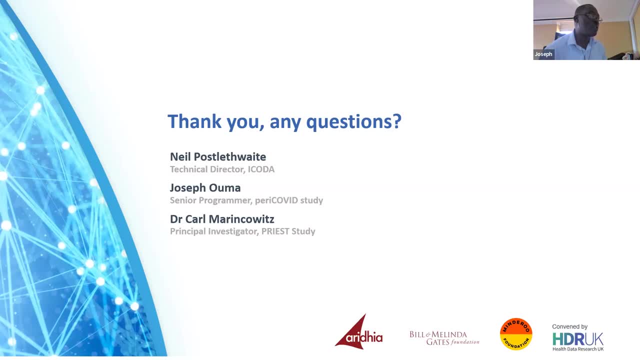 of the secure environment in which this data was being processed And also being able to use the summary data that we were getting out of the dashboard to help their daily work in making decisions about services. So, in general, yes, there was quite a lot of interest. 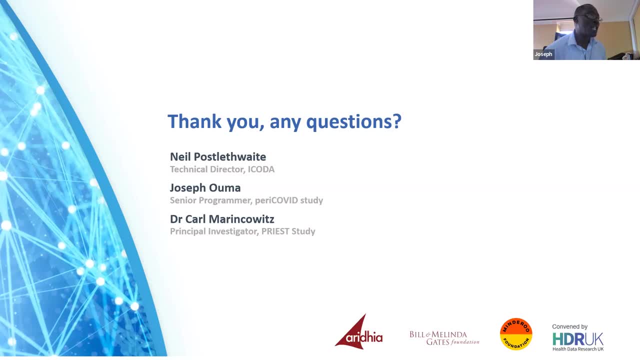 and a lot of engagement with them And they were quite concerned about that security, the patient data security and confidentiality issues, But at the end of it they were quite happy to be able to, you know, use the data and the things that we developed out. 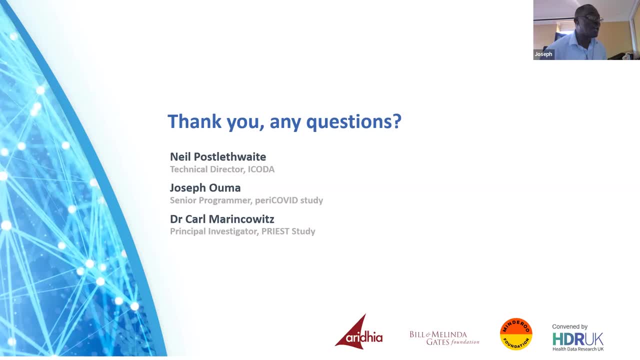 with the data- that's the dashboard- with confidence. I think that was a very good experience and it informed our process all through to ensure that whatever we were leaving behind was acceptable to them, And they were excited about how it's going to help their service delivery. 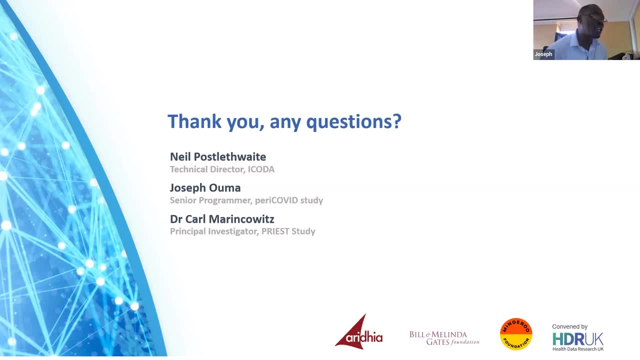 experience in the hospital. I hope that helps. Thank you, It does, Joseph. Thank you, And similarly to Carl, anything that you would call out in terms of privacy considerations from within any of your stakeholder meetings? Yes, So I think. engagement for the PPI group in Sudan. 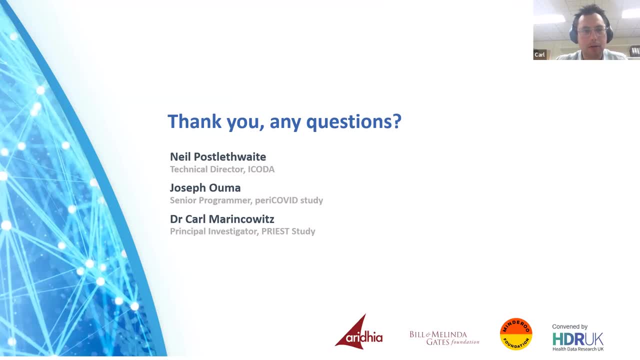 But in South Africa we've established quite a PPI group And we had a longstanding PPI group associated with the priesthood in the UK And data security is a concern for patient stakeholders, especially because of all the things kind of in the news. 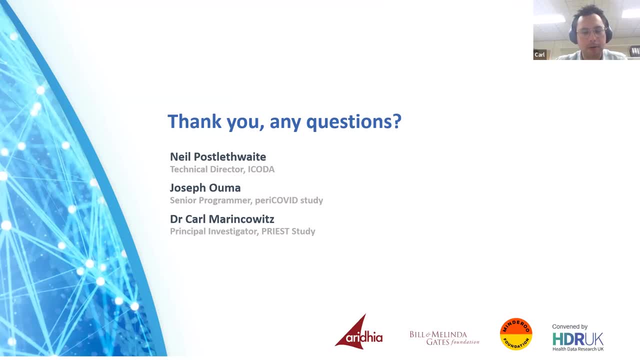 which they hear. But when you generally explain to people that data is anonymized, that it's for a good cause and you can reference that you've got a robust plan for data security generally, PPI stakeholders are happy with that. That was something when we initially applied to ethics. 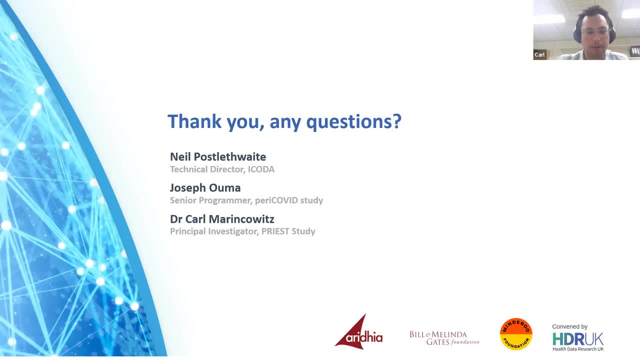 we could go back to them and say that we consulted our PPI group and these are our thoughts. So that was quite helpful. Thanks, And I guess the trusted research environment angle helped a little bit in that discussion. Yeah, it did Perfect. 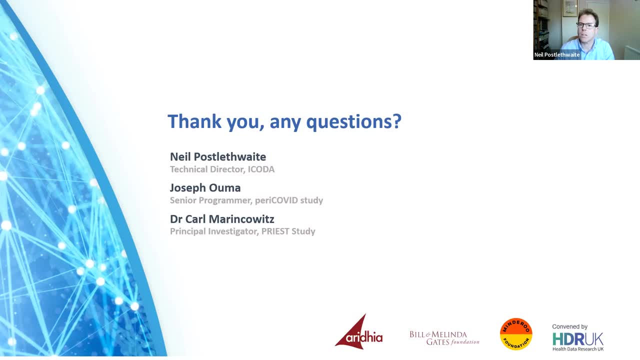 Perfect, Good set of questions And a thank you in the chat for Joseph from James. Any other questions from any of the audience? OK, Well, Let's see. Look, I think that was you know. I'll wrap us up. 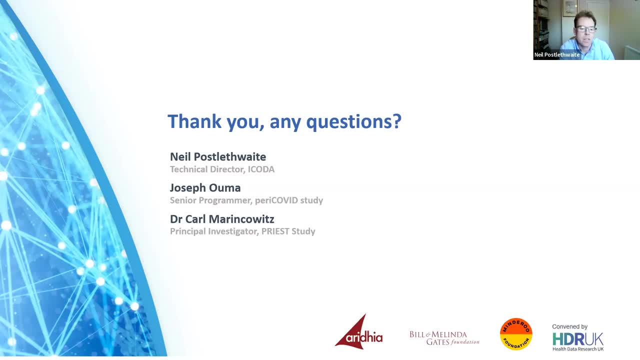 That was a really great and interesting session, So thank you. Thank you to both Joseph and Carl for their fantastic presentations. Really exciting to hear the real use of trusted research environments. A huge thank you to all of our wonderful ICoda researchers right across the globe as they wrap out. 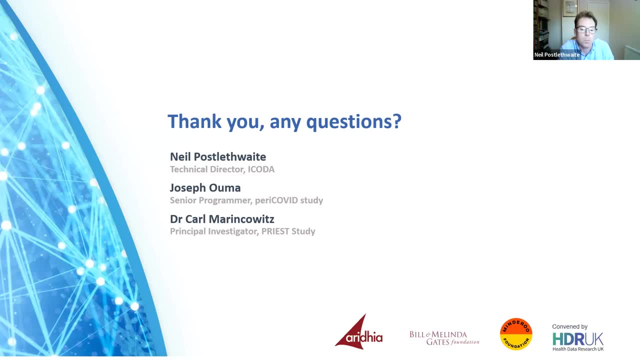 some fantastic projects. OK, Big thank you to our technical partners: Aridia Informatics, who provide our trusted research environments, MMS Holding, who've done data curation for some of the projects, and the SAIL Data Bank, who've provided storage. 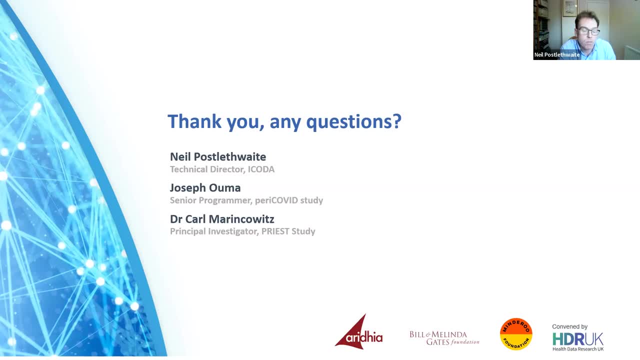 and part of the federated analysis solution. Our funders- the Bill and Melinda Gates Foundation, Mindaroo Foundation and Microsoft AI for Health, Health Data Research UK. our convener- obviously, my colleagues in the ICoda program. Without you, we wouldn't all be here. 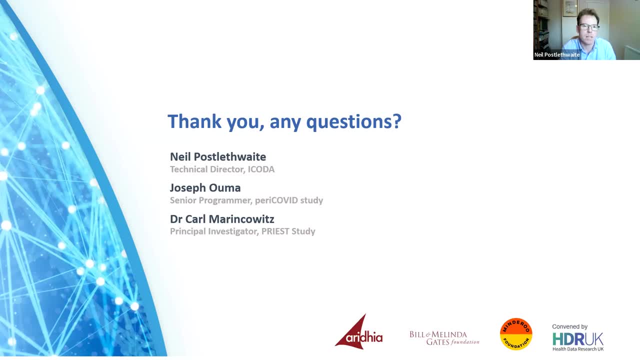 And thanks to all of you in the audience for taking the time to learn a little bit more in terms of trusted research environments and the experiences using them in what's a very exciting space as we look at privacy-enhancing technologies going forward. Thank you all. 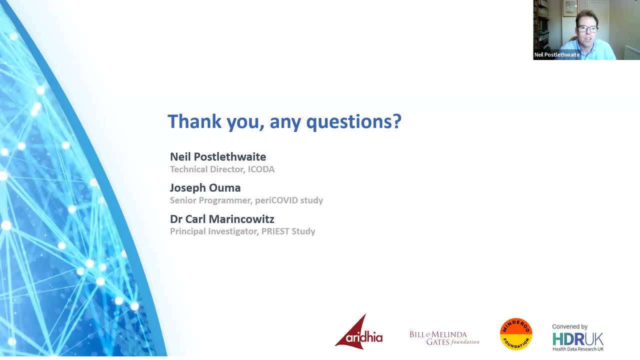 Have a fantastic day. Thanks Carl, Thanks Joseph, Thank you.